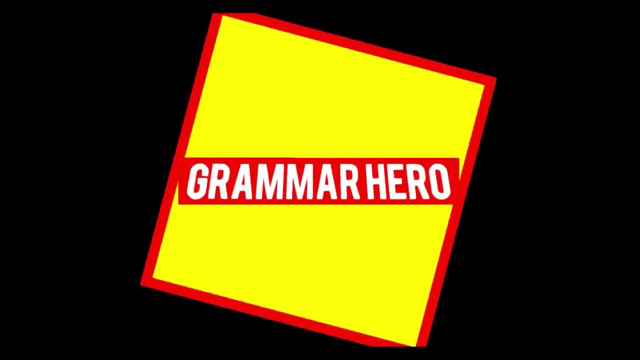 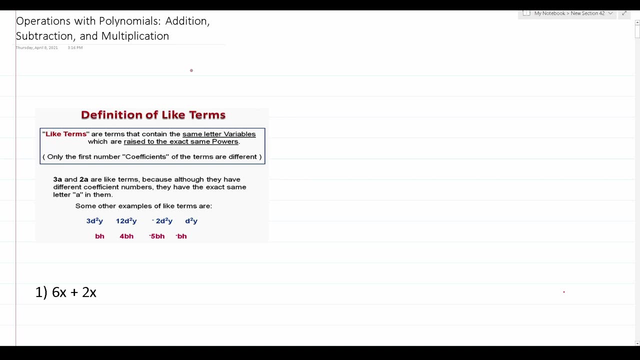 Welcome YouTubers to another episode in my Grammar Hero series. In today's video, I'm going to be discussing how to perform operations with polynomials. More specifically, I'm going to focus on adding, subtracting and multiplying polynomials. As you can imagine, this is a topic. 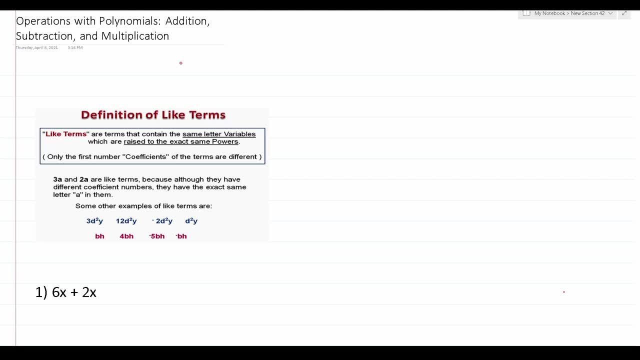 that frequently appears on the ASVAB. That said, I realize that some of you are pretty good at math already, so in the description of this video I also included time stamps, and those time stamps are associated not only with the topics that I'm discussing in today's video, but also with 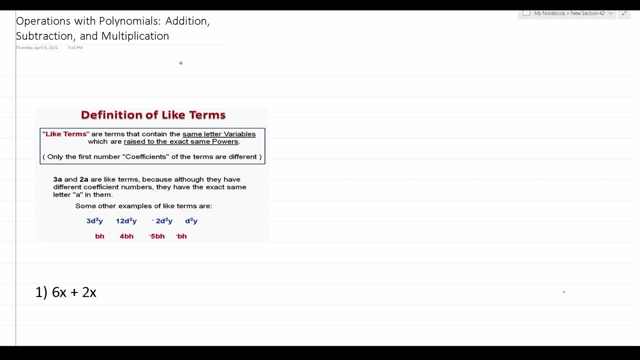 the practice questions in today's video. In total, there's 22 practice questions in today's video. so if you're good with polynomials, what you can do is you could just click on those time stamps, work out the practice problems and move on. Otherwise, again, it's in your best interest to watch this video from start to finish. 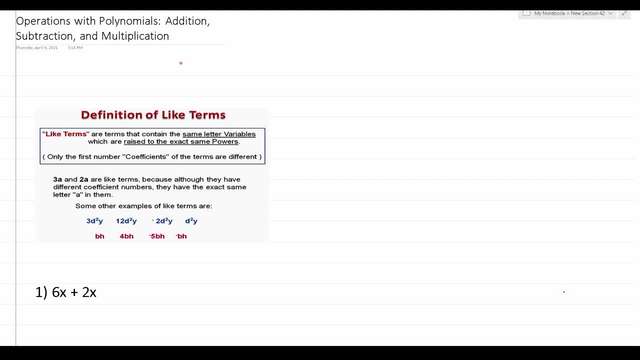 and, moreover, you should pause the video whenever I get to a practice problem, attempt to work it out on your own and then resume playing the video to check your solution. So, all that being said, let's go ahead and get started with today's video. All right, so prior to performing any 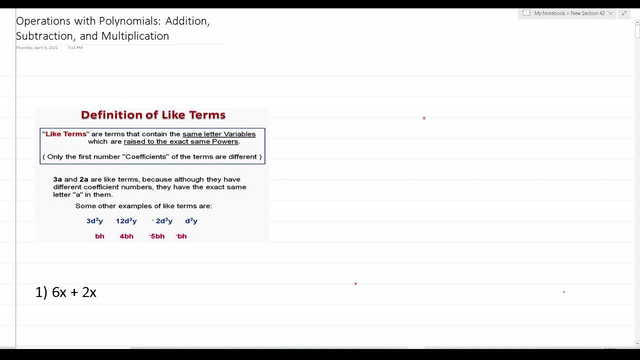 operations with polynomials, we do have to review one very important concept, notably the concept of like terms. and, as you can see, I put the definition of like terms here to start, and it says: like terms are variables that contain the same letter, variables which are raised to the same exact power. So again, like terms are: 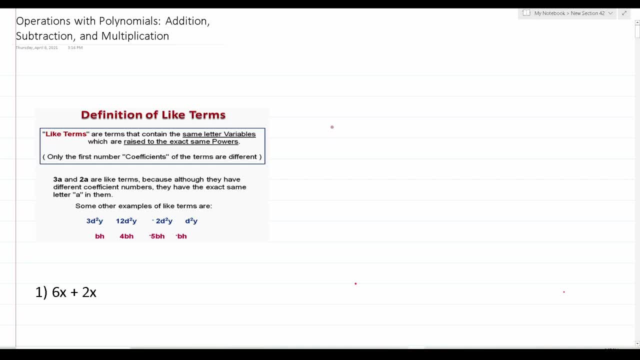 terms that contain the same letter variable, which are raised to the same exact powers. So, for example, let's take a look at two terms, notably 3a and 2a. Are those like terms? Well, they have the same letter variable. in 3a, our letter variable is a and in 2a, our letter variable is a as well. Likewise these: 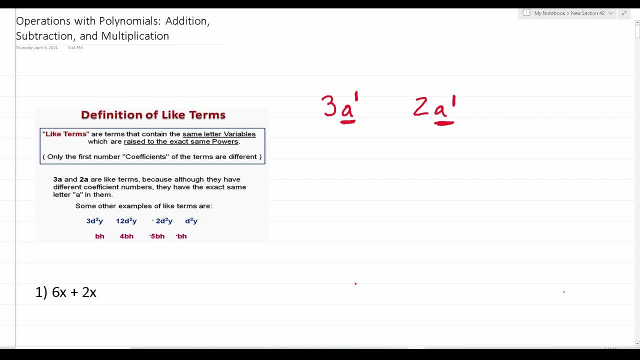 are both raised to the first power. therefore, they are like terms, and one thing you can do with like terms is you can add and subtract them. So 3a plus 2a would be 5a. So let's take a look at another example. 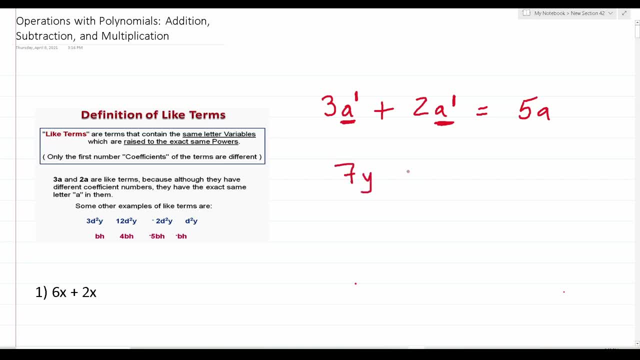 let's say we had 7y plus 10x squared. Are these like terms? Well, our letter variables in 7y is y and our letter variable in 10 x squared is x. Those letter variables are not the same, so are not like terms and therefore we could not add them. All right, let's look at one more example. 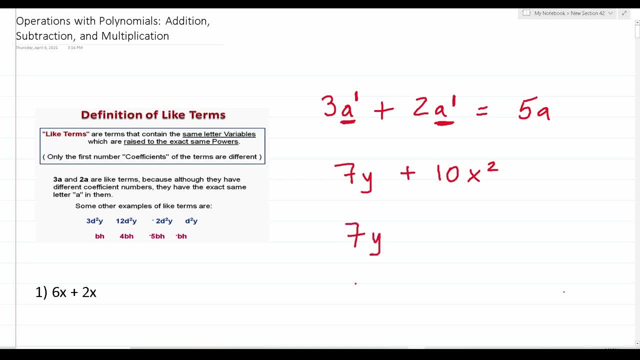 Notably, let's say we had 7y squared plus 7y. All right, according to the definition of like terms, a like term has the same letter variable. So in 7y squared our letter variable is y and in 7y our letter variable is also y. With that said, the second part of the definition says: 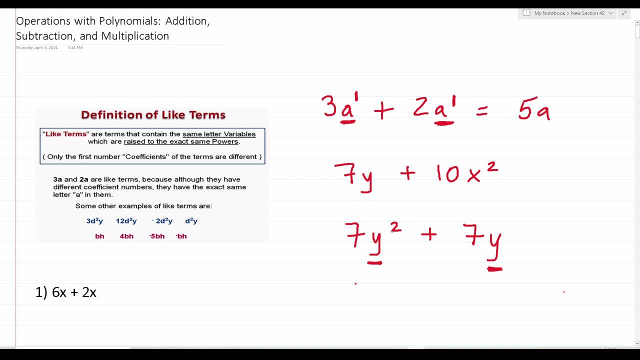 they have to be raised to the same exact powers. In 7y squared, our power is 2, whereas in 7y, our power is 1.. In light of the fact that they have different powers, these are not like terms. 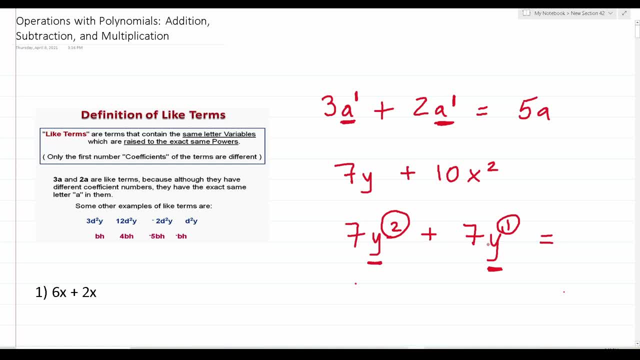 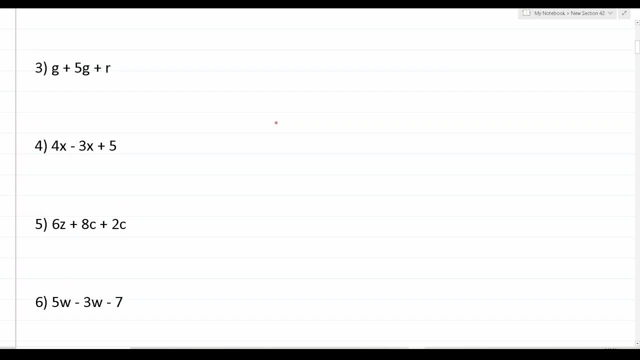 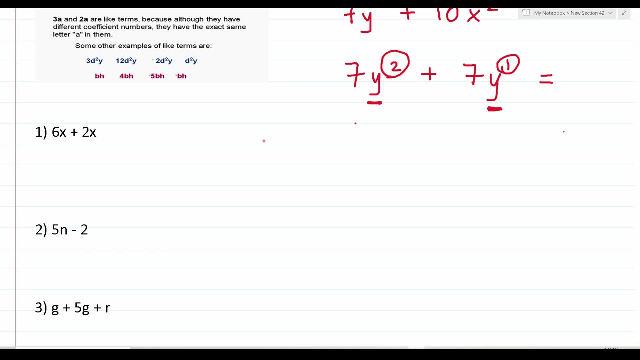 and therefore we wouldn't be able to add them together. So, with that in mind, let's go ahead and take a look at these 10 practice problems. Again, these are very simple problems, just to get you comfortable with identifying like terms and, beyond that, adding or subtracting them. very 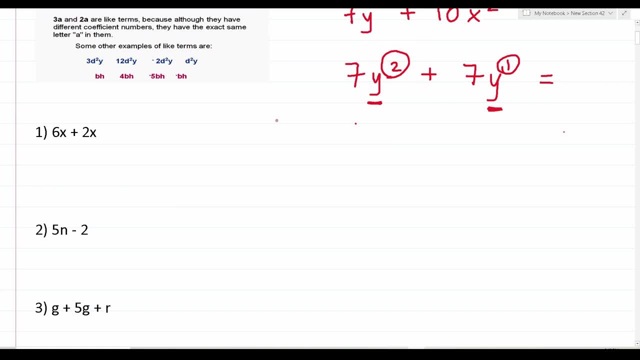 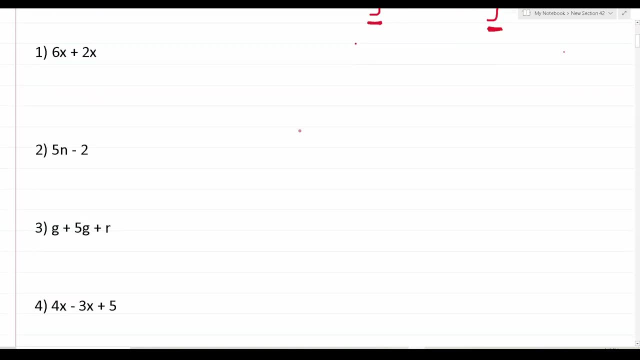 quickly. So if, at this point, you want to pause the video and work out these problems on your own, that's a good idea. Again, these problems are very, very simple. So this first one says 6x plus 2x. Again, according to the definition, a like term has the same letter variable. 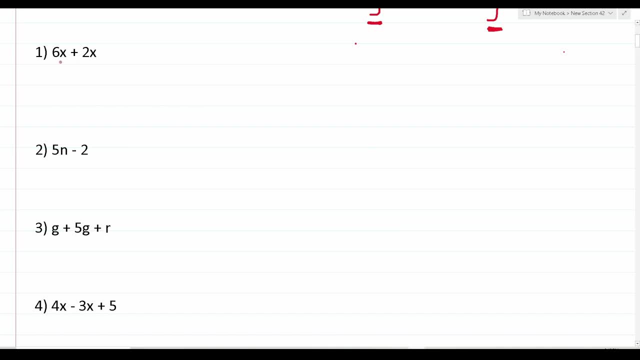 As well as the same power. So in 6x our letter variable is x and in 2x our letter variable is also x, Even though it's not expressed. you should know that these are raised to the first power. 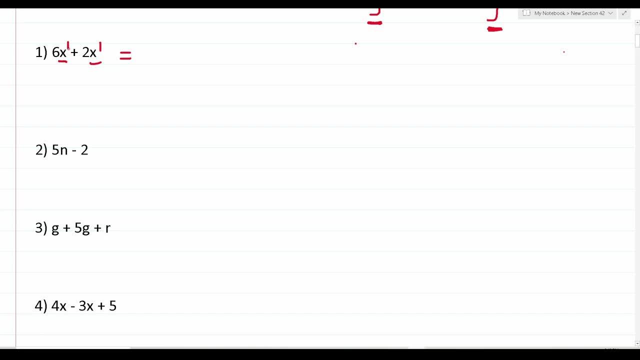 and in light of the fact that these have the same letter variables and are raised to the same exponents, we can add these together: 6x plus 2x is going to be 8x, And you may have noticed that it doesn't matter what comes in front of the letter variable. 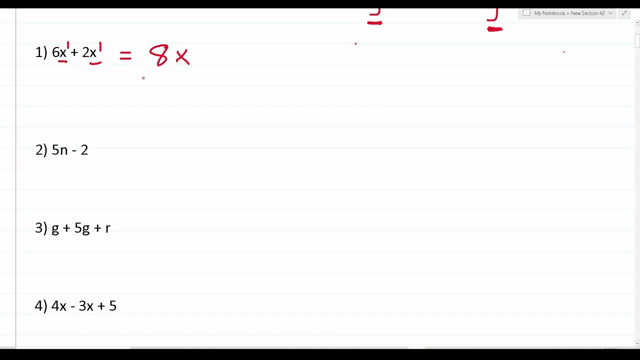 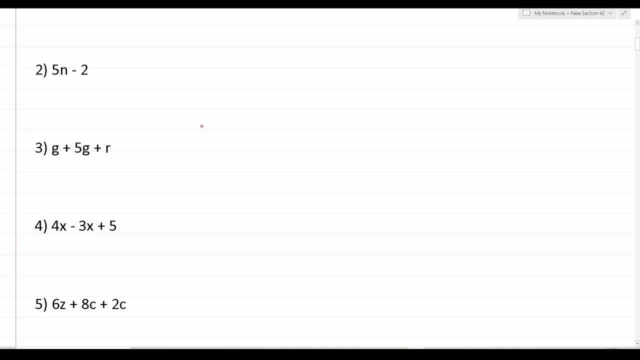 Those are called the letter variables and those are called the letter variables. These are called coefficients and, as you just saw, we're simply adding those together. All right, let's look at number 2 now. It says 5n minus 2.. Again, according to the definition, 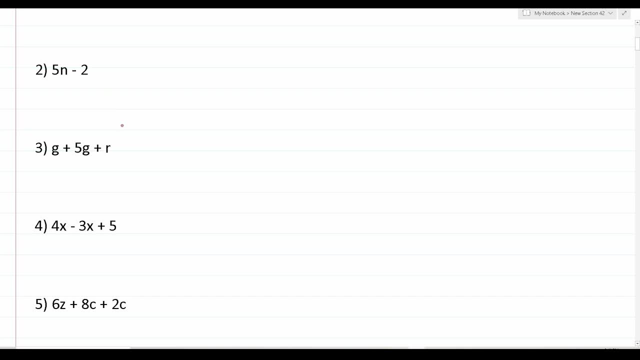 for these to be like terms, they have to have the same letter variable and they also have to be raised to the same power. So in 5n our letter variable is n and in 2, we have no letter variable. So in light of that, these are not like terms and therefore we can't perform this. operation. So we're going to have to add these together. So we're going to have to add these together. So, in light of that, these are not like terms and therefore we can't perform this operation. So, in light of that, these are not like terms and therefore we can't perform this. 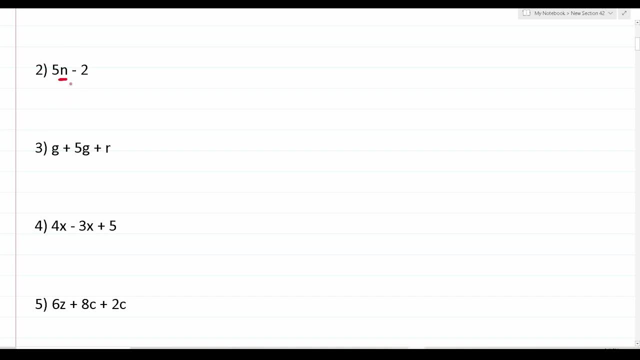 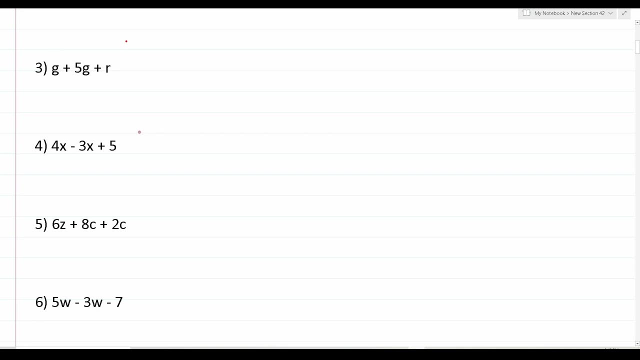 operation. So, in light of that, these are not like terms and therefore we can't perform this. So, in other words, this one is as simplified as it's going to get All right. so if we take a look at number 3, it says g plus 5g plus r. Let me just stress this. 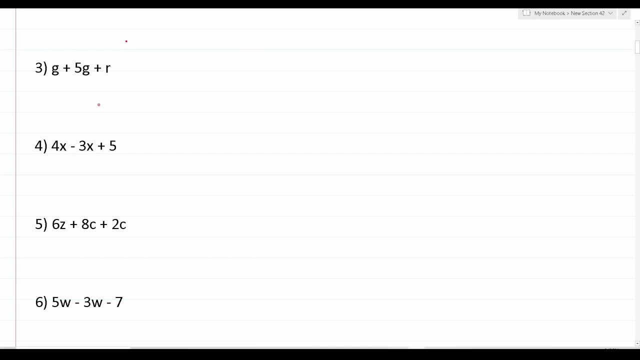 and I'm going to rewrite this over here so it's more clear: Whenever the coefficient's not expressed in front of a variable, it's implied that it's 1.. So you can regard this as 1g plus 5g plus 1r. 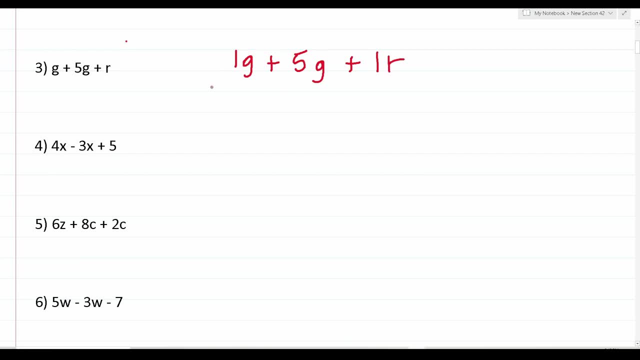 again. typically that one is not expressed. as a matter of fact, when we simplify this one, we're going to get rid of it. so again, according to the definition, like terms have to have the same letter variable as well as the same power. so in 1g we have the letter variable g and it's raised. 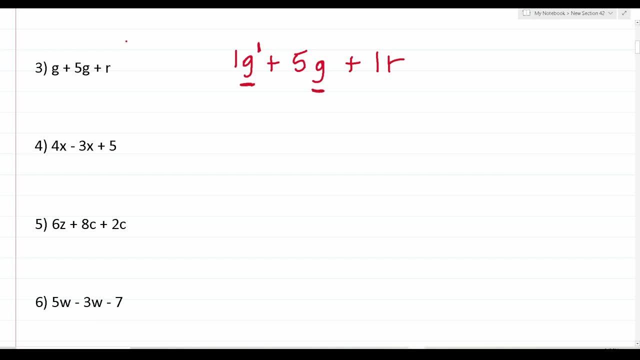 to the first power. in 5g we have the letter variable g and it's raised to the first power, and here we have the letter variable r. so, as we can see, like terms are 1g and 5g and 1r is not a. 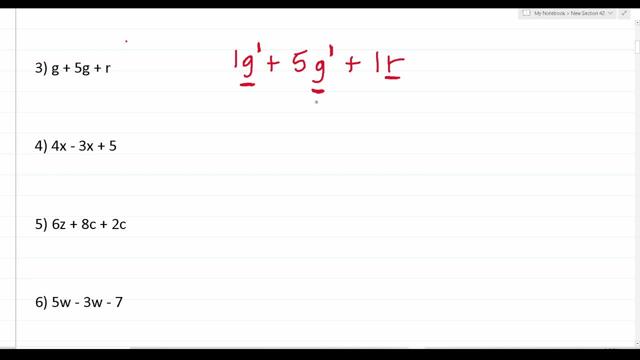 like term of those. so in light of that we can add 1g and 5g together. 1g plus 5g is going to be 6g and we'll just tack on this and I'm going to drop this one because it's implied. 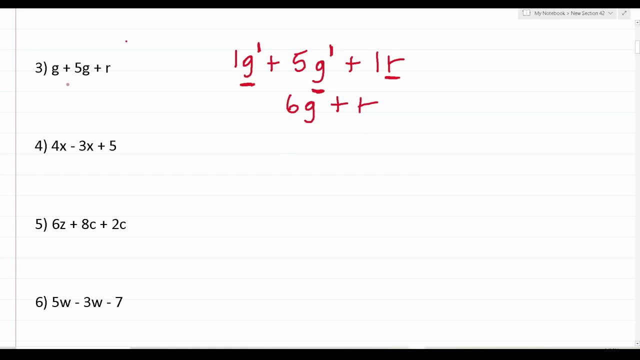 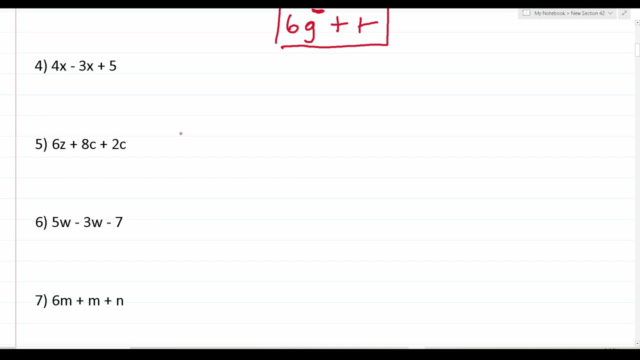 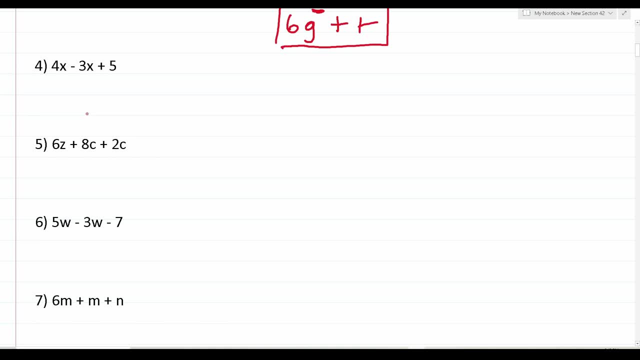 according to the definition, for these to be like terms they have to have the same letter variable as well as the same power. So we have our letter variable x raised to the first power. We have our letter variable x raised to the first power. So those two. 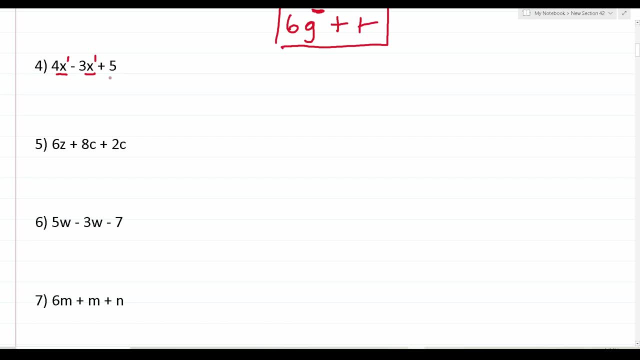 are like terms, Then we just have 5 with no letter variable, so it's not a like term. When we have like terms, we can perform the operation. So we could do 4x minus 3x, which will just leave us with 1x or x plus 5.. Alright, so that's that one, Pretty easy. 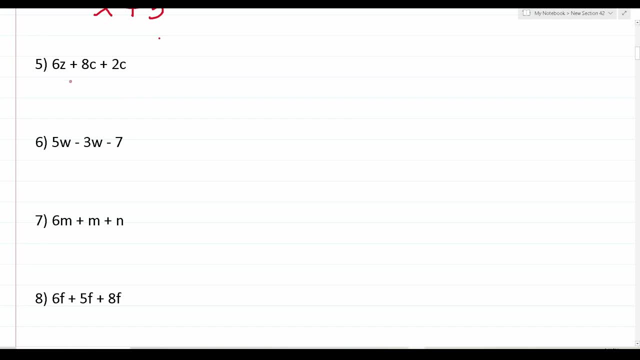 Let's move on to number 5.. We have 6z plus 8c plus 2c. Again, according to the definition, for these to be like terms they have to have the same letter variable And be raised to the same power. So we have letter variable z here, raised to the first. 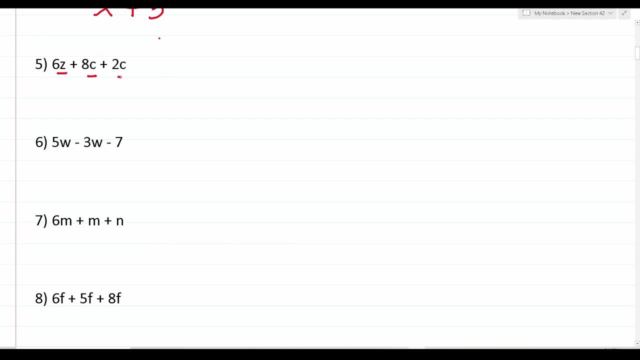 power Letter: variable c raised to the first power Letter. variable c raised to the first power. So whereas 8c and 2c are like terms, 6c isn't. So again, when we have like terms, we can add and subtract those terms. So in this case we can do 8c plus 2c, which is 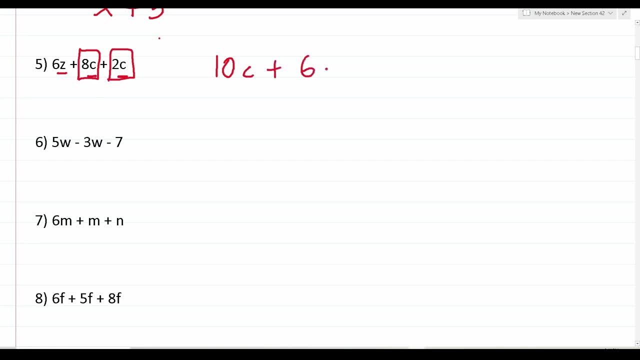 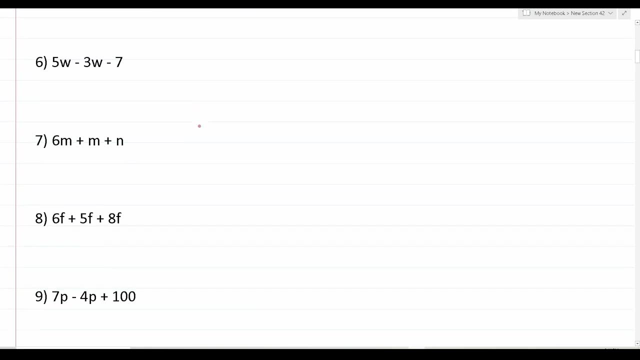 10c plus 6c z, And again, we couldn't add 6c to 10c because it's not a like term. Alright, let's keep working these out. We have 5w minus 3w minus 7.. Again, according to the 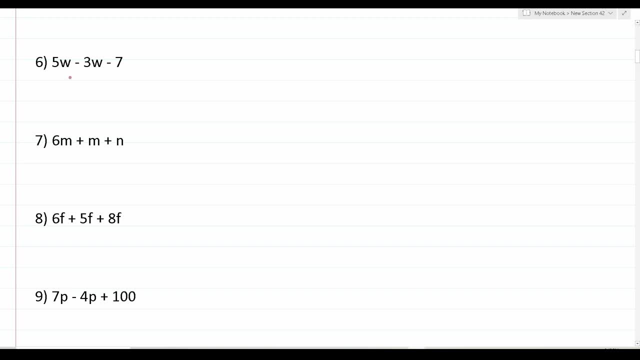 definition. they have to have the same letter variable as well as the same power in order to be like terms, And then, if they are like terms, you can add and subtract them Again. we have w here, w here, First power here, first power here, Whereas we have 7 here with no letter. 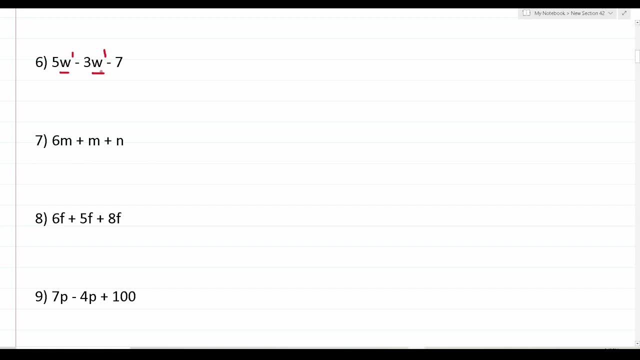 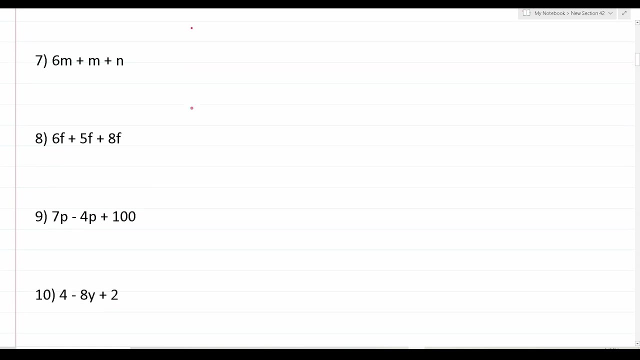 variable. So 5w and 3w are like terms. Therefore we can perform this subtraction: 5w minus 3w is 2w, and then we'll just tack on that minus 7.. Alright, let's keep working these out. We have 6m plus m plus n. So again, according to the 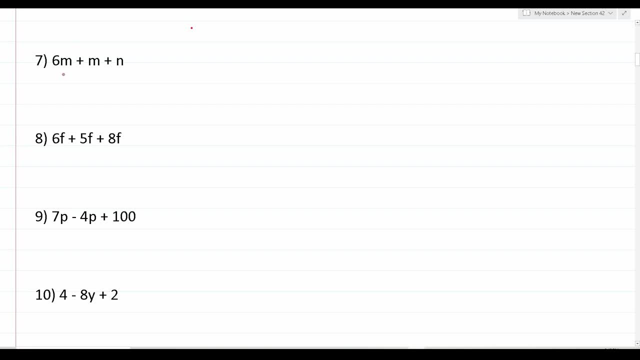 definition they have to have the same letter variable as well as the same exponent in order for us to add like terms. So here we have the letter variable m. It's raised to the first power. We have the letter variable m raised to the first power. We have the letter variable n. So 6m and m are like terms, n. 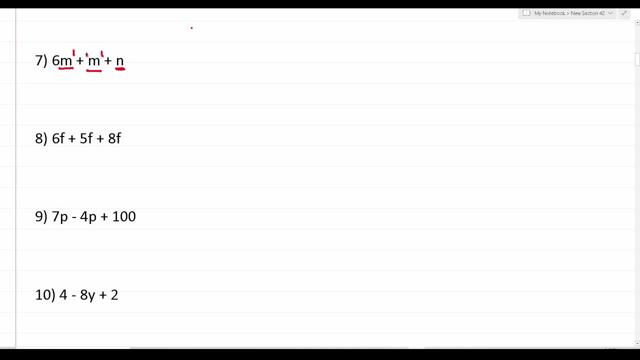 is not. So, again, if it's not expressed, there's always an imaginary 1 there, So let's go ahead and rewrite this off to the side, if we need to. This is 6m. Let me fix that real quick. 6m plus. 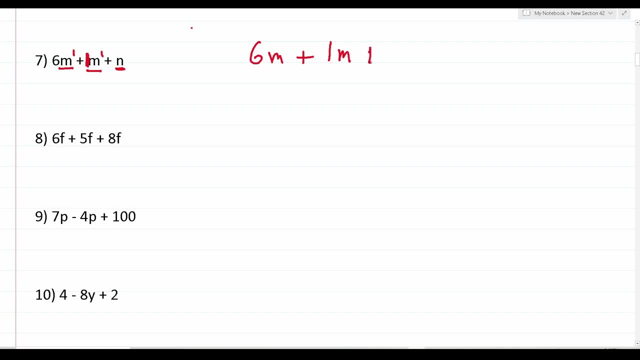 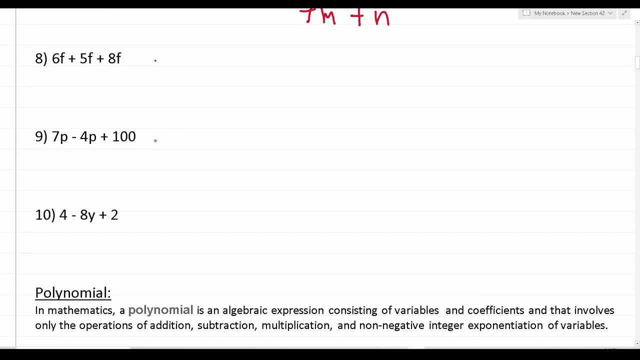 1m plus n. 6m plus 1m is going to be 7m plus n, And we can't do anything else since 7m and n are not like terms. Alright, number 8 says 6f plus 5f plus 8f. Again, if they're like terms, we can. 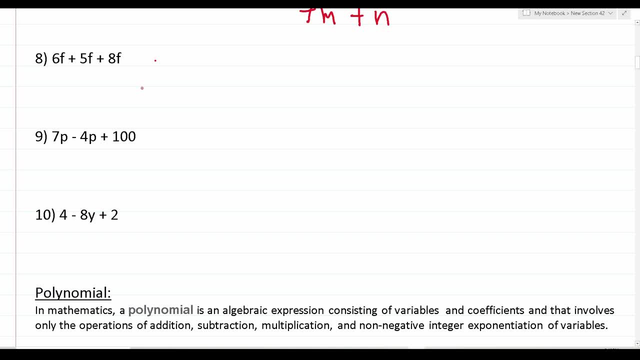 perform that operation of addition. If they're not like terms, we can't, And according to the definition, like terms have the same letter variables raised to the same powers. So we have 6f here. Our letter variable is f. It's raised to the first power. That's implied. We have 5f. 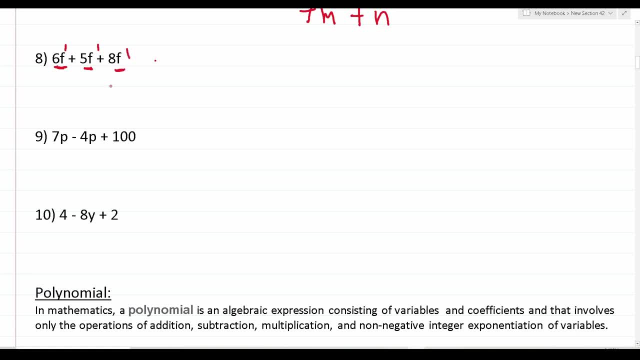 raised to the first power, We have 8f raised to the first power. So clearly these are all like terms So we can add them all together. So 6 plus 5f is going to be 11f. 11f plus 8f is going. 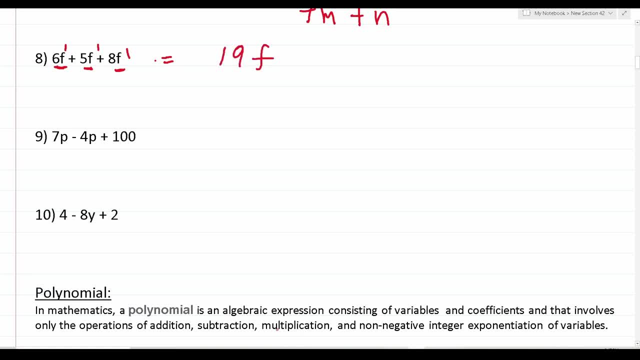 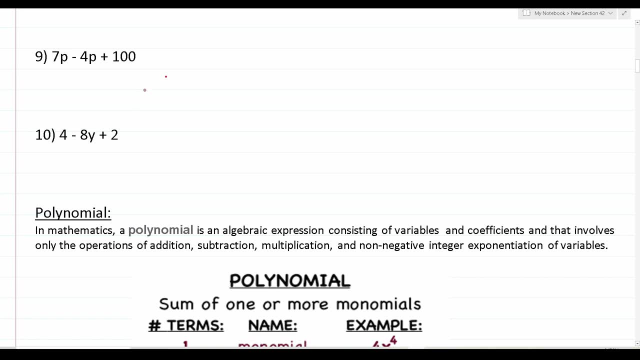 to be 19.. All right, So number 9 says 7p minus 4p plus 100.. Again, clearly, 7p and 4p are like terms, given that they have the same letter variable of p, And those letter variables are raised to. 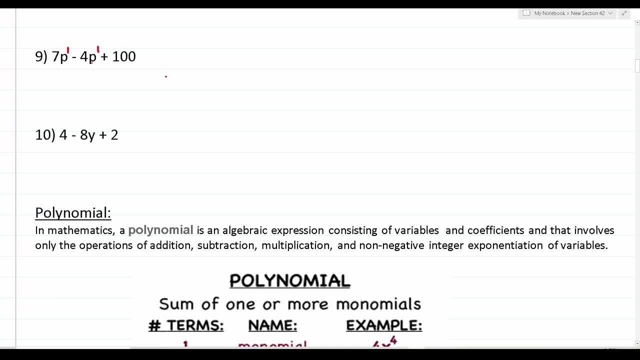 the same power. So we can perform this operation of 7p minus 4p, But we can't do anything with this plus 100 because it's not a like term. So 7p minus 4p is going to be 11f And we can't do. 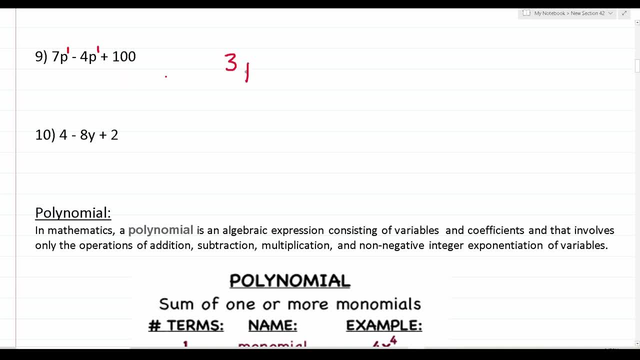 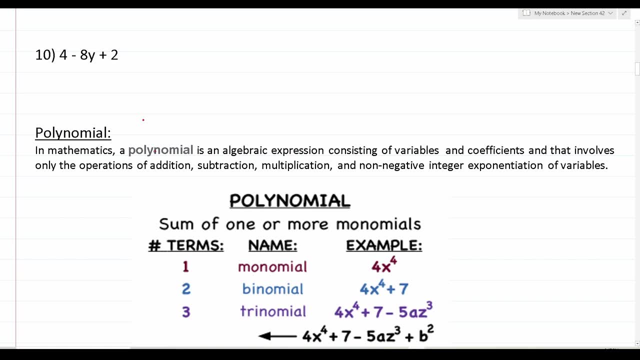 anything with this plus 100, because it's not a like term. So 7p minus 4p is going to be 11f, All right. And finally, number 10 says 4 minus 8y plus 2. We should be able to tell that 4 and 2. 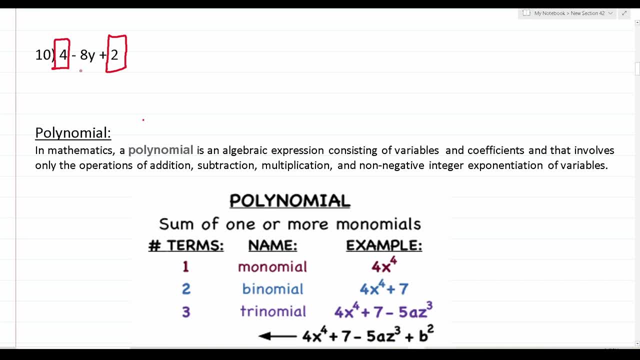 are like terms, whereas negative 8y is not a like term. So we'll perform 4 plus 2, which is going to be 6 minus 8y, And we're done with that one. So now that we've reviewed, 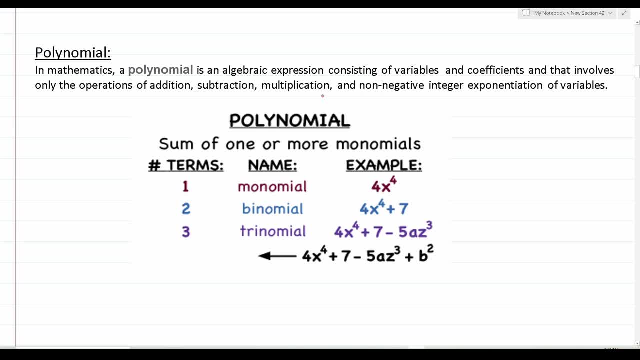 the definition of like terms, as well as worked out some very basic examples involving operations involving like terms. let's go ahead and start talking about polynomials More specifically. let's review the definition of what a polynomial is. For some reason, a lot of people struggle with. 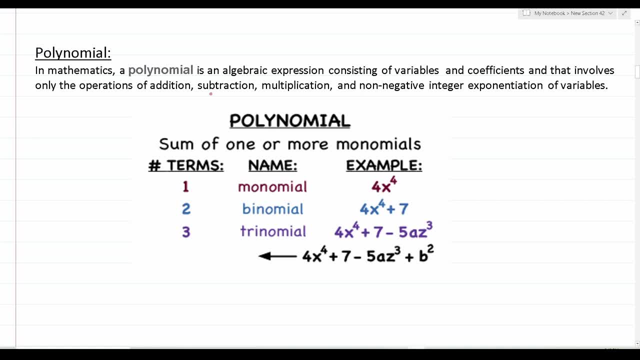 understanding what a polynomial is, But hopefully this definition makes it very simple and straightforward. So our definition here says: in mathematics, a polynomial is a number of variables. A polynomial is an algebraic expression consisting of variables and coefficients that involves only the operations of addition, subtraction, multiplication and non-negative. 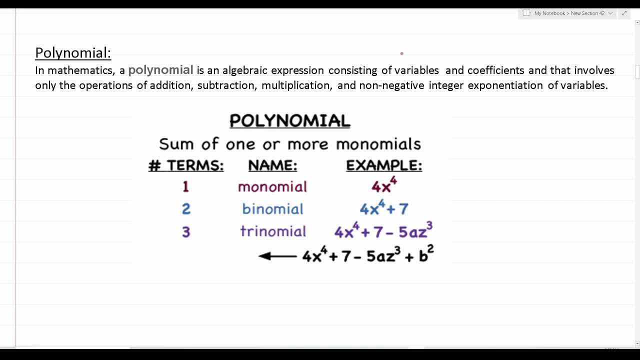 integer exponentiation of variables. Well, while it's easy to understand addition, subtraction and multiplication, what does non-negative integer exponentiation of variables mean? It means that the power to which you raise the variable is the power to which you raise the. 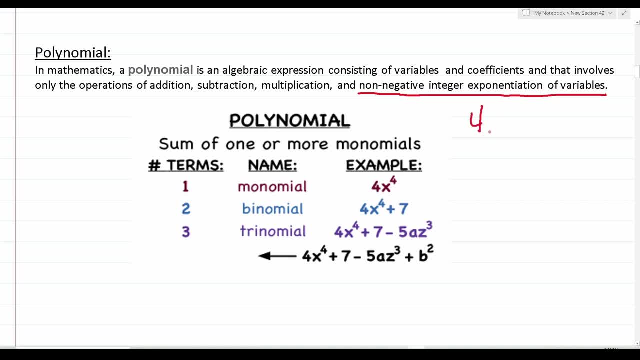 variable can't be negative. So if we have 4x squared, that is a polynomial. If you have 4x to the negative 2, that integer is negative. Therefore, this is not a polynomial, It's something else. Okay, so again, non-negative integer exponentiation, which I like the sound of. 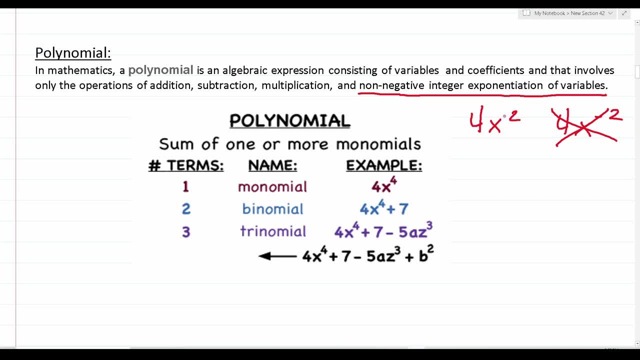 just means that the exponent has to be positive. So in all the examples you're going to see today, all the exponents are going to be positive, All right. that said, polynomials have different classifications, and let's take a look at that. 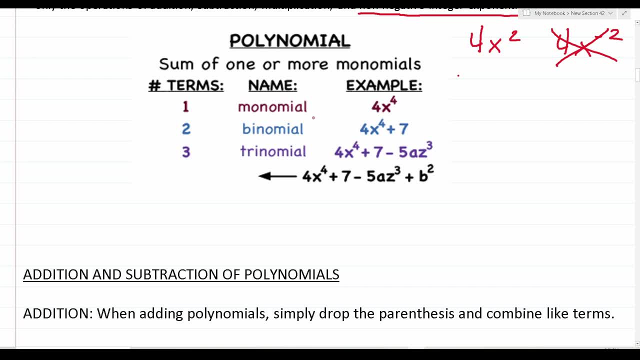 because I think a lot of people get these confused, even though they're pretty simple. A polynomial that only has one term, such as 4x to the 4th, is what's referred to as a monomial, A polynomial with two terms, such as: 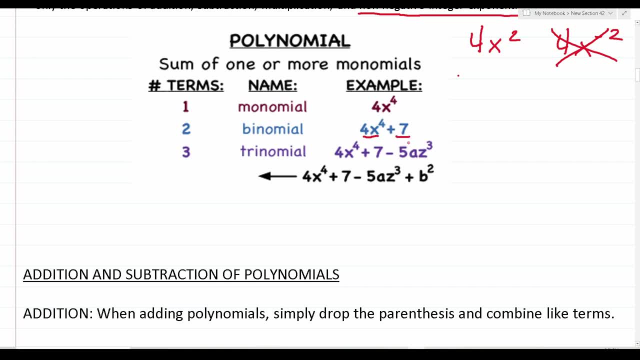 4x to the 4th plus 7.. Again, this is one term. This is the second term is what's called a binomial, A polynomial that has three terms, such as 4x to the 4th plus 7, minus 5az to the 3rd. Again. 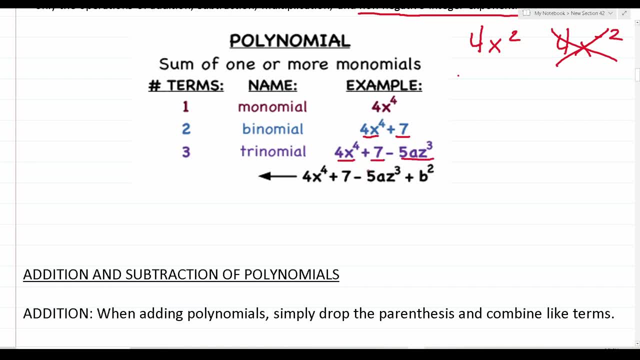 here's our first term. second term, third term is called a trinomial, And a polynomial that has four terms, such as 4x to the 4th, plus 7, minus 5az to the 3rd, is called a trinomial. 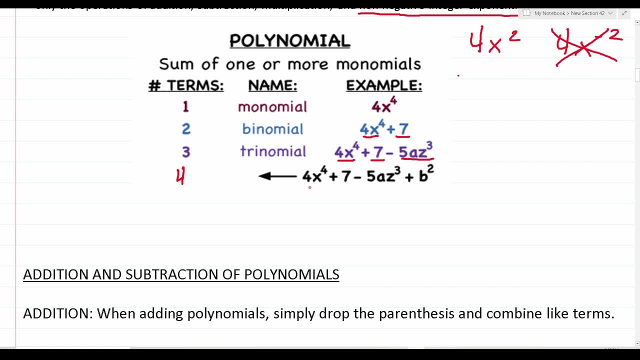 Plus 7 minus 5az to the 3rd plus b. Again, here's our four terms: 1, 2, 3, 4, is called a quadrinomial, All right, so again, if you ever see these terms- monomial, binomial, trinomial. 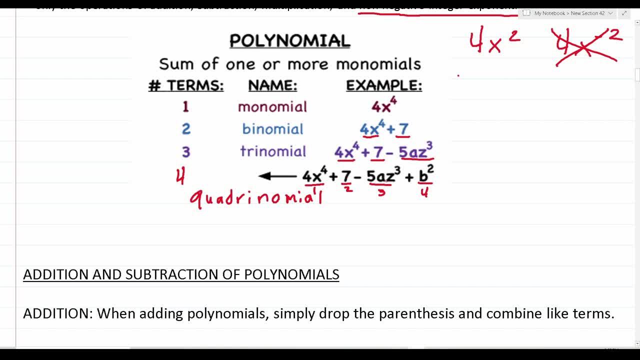 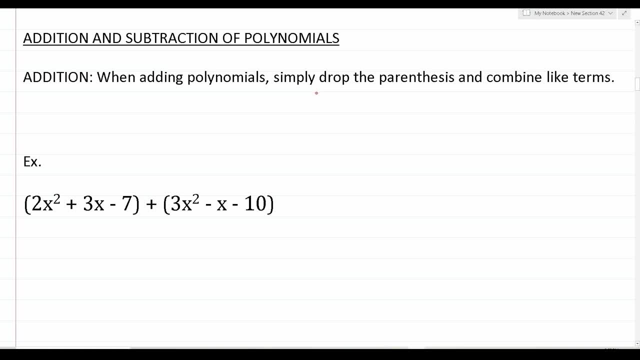 quadrinomial. again, that's just telling you how many terms there are in a polynomial. There's nothing more to it than that. All right. so with our knowledge of the definition of like terms, as well as our knowledge of polynomials in mind, let's go ahead and work on adding and subtracting polynomials. 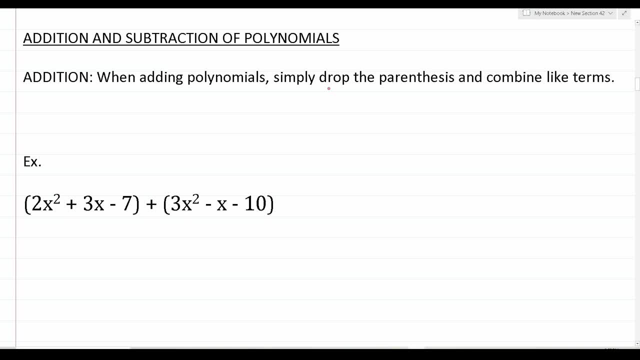 And, as I stressed at the beginning of this video, this is very, very simple to do. So. in order to add polynomials, you simply drop the parentheses and combine like terms. Well, that's pretty simple to do, So let's look at an example. 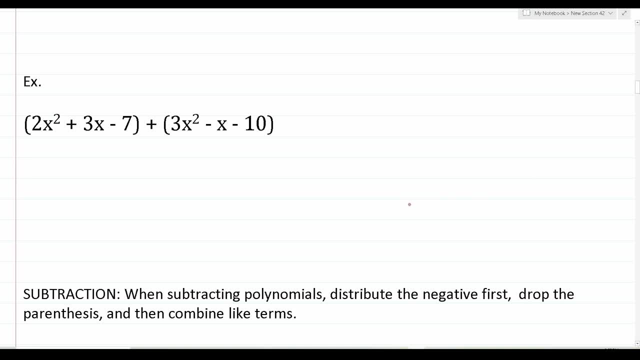 So in this example we have 2x squared plus 3x minus 7, all in parentheses, plus, in parentheses, 3x squared minus x minus 10.. Again, to add polynomials, drop the parentheses and then combine like terms. So let's go ahead and do that, And I'm going to do that up here. 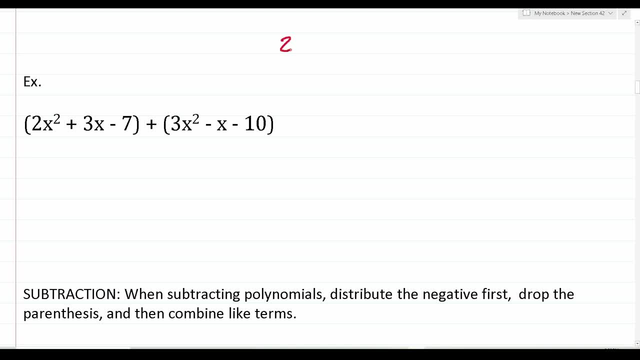 So the very first thing I'm going to do is drop these parentheses. We have 2x squared and I'm going to do that up here. So let's go ahead and do that, And I'm going to do that up here. 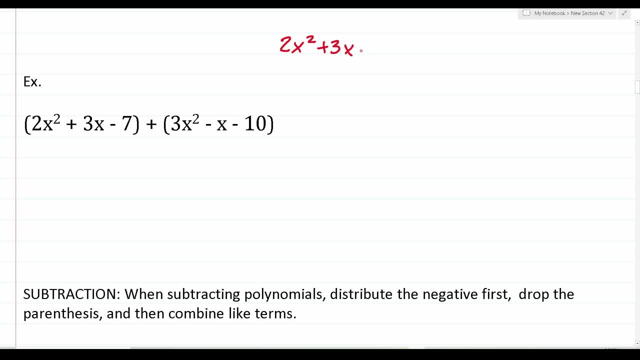 squared plus 3x minus 7 plus 3x. squared minus x minus 10.. Again, we just dropped those parentheses. Now we're looking for like terms that we can combine. Again, the definition of like terms is same letter variable raised to the same power. So if we look at our first term here, 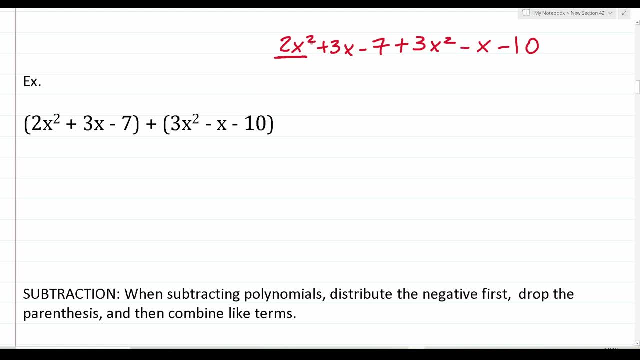 we can see that we have the letter variable x raised to the second power. We look through all these other terms. Do we have anything else that meets those two criteria? Well, this is x raised to the first power. This is just negative 7. But here we have x raised to the second power. So 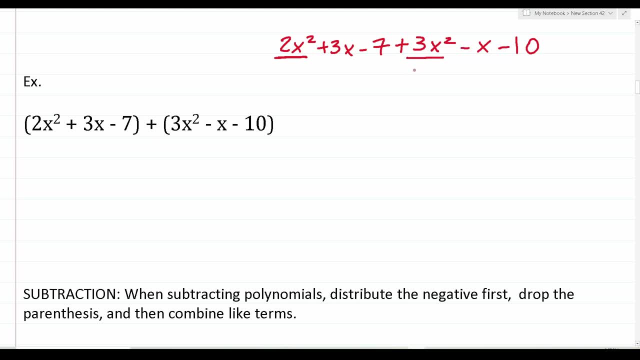 3x squared and 2x squared are like terms And therefore we can combine them. 2x squared plus 3x squared, x squared is five x squared, and now that we've combined them, let's go ahead and just cross them out. that way, this uh polynomial looks a little bit easier to work with. all right, so moving on. 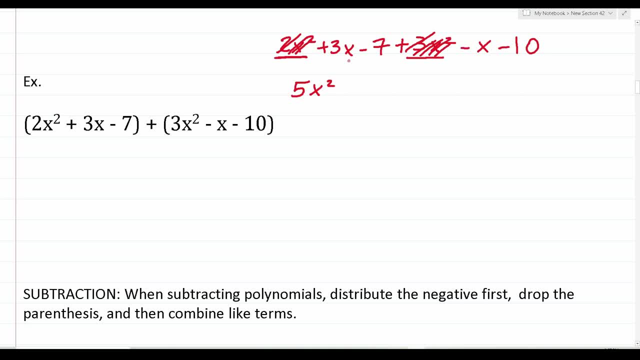 to the next one. we have three x again. our letter variable is x and it's raised to the first power. we look through the rest of these terms. do we have anything else? that's, uh, a like term. well, this is just negative seven. but here we have x and again it's raised to the first power. so 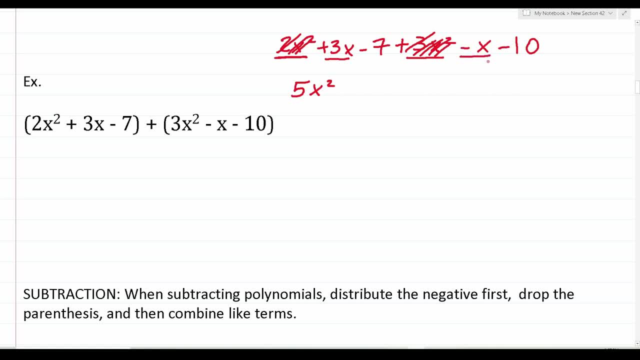 uh, three x and this negative x are like terms, therefore we can combine them: three x minus x is just going to be two x, and now that we've combined them, we can simply cross them out here to make this a little bit easier. and then finally, uh, we have minus seven and minus ten, which are 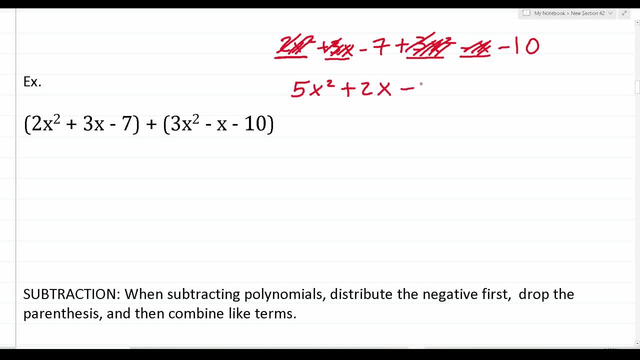 like terms, uh, minus seven and minus ten, which are like terms minus seven and minus ten, which are like terms minus seven minus ten is minus seventeen, and just like that we're done with this one. we took these uh, two polynomials and we added them together. more specifically, we dropped the parentheses. 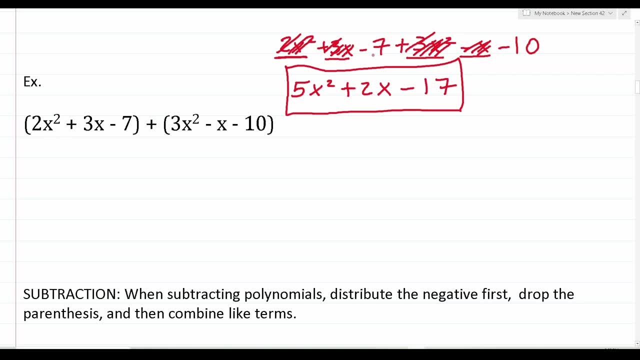 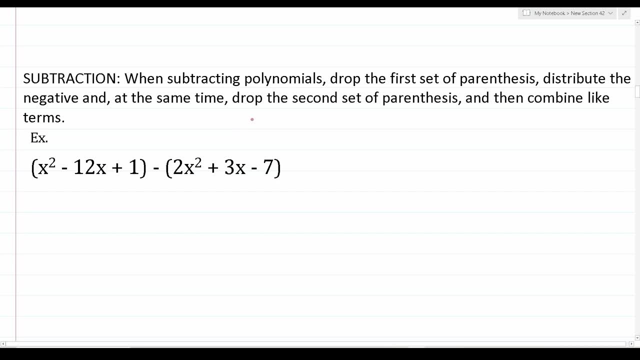 and then we just went through and combined the like terms. there's nothing more to it than that. all right, so as far as subtracting polynomials goes- uh, it's very similar to adding polynomials. that said, we go about dealing with our parentheses as well as our subtraction sign, uh, in a different way. 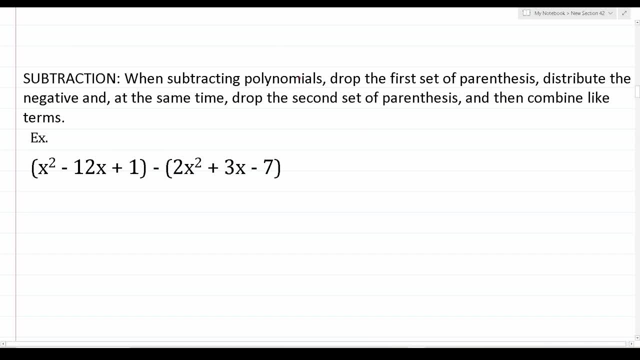 and if you're the type of person who likes instructions, here they are. says: when subtracting polynomials, drop the first set of parentheses. so that would be these here. distribute the negative. so here's our negative. it's a subtraction symbol. we're going to distribute it here, here and here. 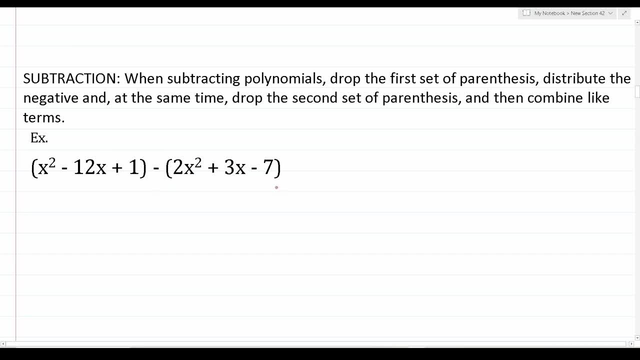 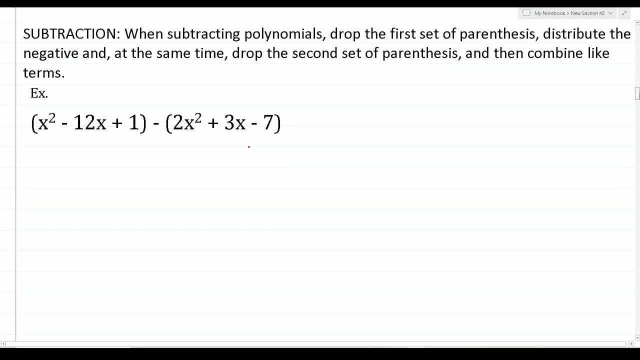 and at the same time drop the second set of parentheses. so that would be these here, and then combine like terms. so let's go ahead and see what that looks like in practice, and it's not too difficult at all. again drop this first set of parentheses. so let's do that we have. 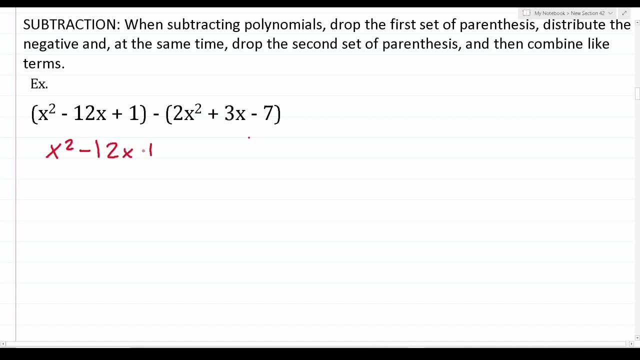 x squared minus 12x plus one. take this negative and distribute it. so we're going to distribute it here, here and then here, and at the same time that you're distributing this negative, go ahead and drop your second set of parentheses. so we have negative times, uh. 2x squared a. negative times a. 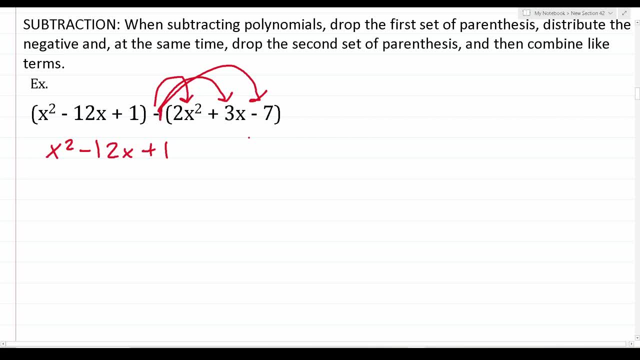 positive is a negative, and if it's helpful, you can imagine that there's a negative one here, and one times anything is just itself. so negative one times positive: 2x squared is negative, 2x squared negative. one times positive: 3x is negative, 3x. and then 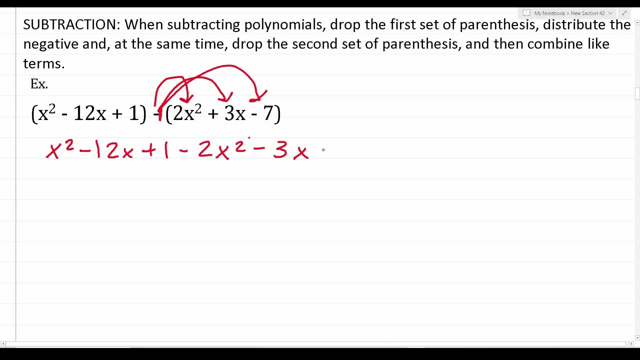 negative. one times negative, 7 is going to be positive 7, given that a negative times a negative is a positive. again, on my channel, i have a video in regard to how to multiply positives and negatives, so if that's something with which you struggle, go ahead and check out that video. 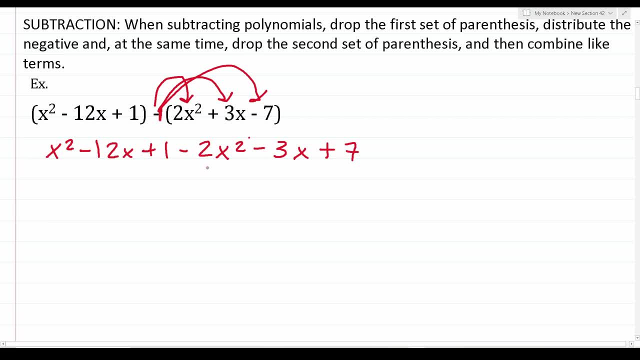 but, that said, let's go ahead and get back to this problem again. we dropped our first parentheses, we took our negative and distributed it, and then we're going to distribute it here and at the same time, we're going to distribute it. at the same time, we dropped our second set of parentheses, so now all we have to do is combine. 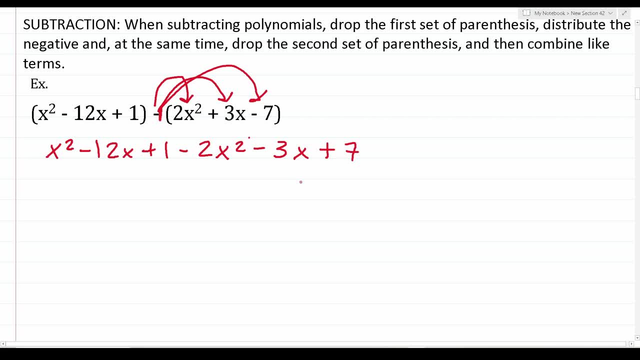 like terms, again like terms. same letter variable to the same power. so if we look at x squared here, we're looking for something with the letter variable x raised to the second power, which is right here. so we have x squared minus 2x squared. that's going to be negative. x squared and again. 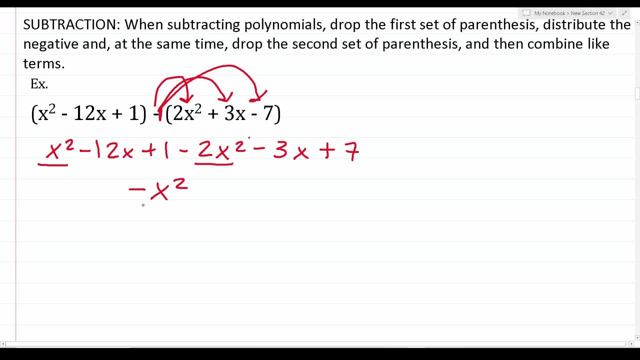 if you can't add or subtract negatives, i'm going to create a video for that very soon. but basically this is the same as negative 2 plus 1. again there's an imaginary 1 here. negative 2 plus 1 is going to be negative 1. 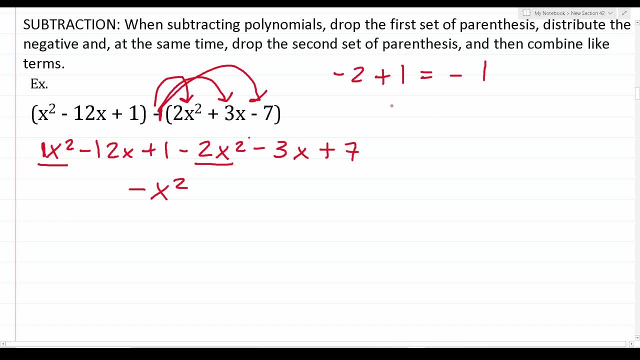 and the way you want to view this. if you can't understand this is you break out your number line. let's say: here's negative 2, this is negative 1, this is 0 and this is 1. so we're starting at negative 2, which is right here, and then we're going to create a video for that very soon. so 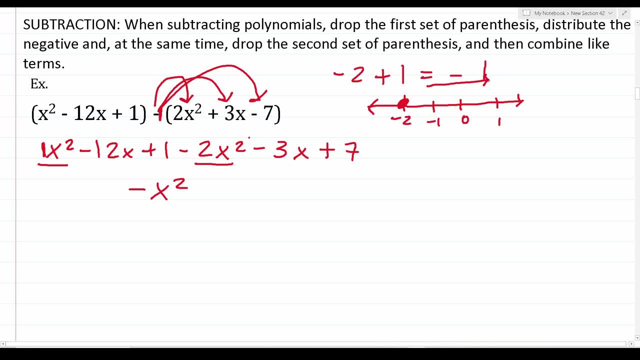 on a number line: when you add, you go this way. when you subtract, you go this way. so this is negative 2 plus 1. so we're going to move to the right 1, which gets us to negative 1. and again we don't express that 1 in front of our variable here, which is why it drops. so again, i'm going to make: 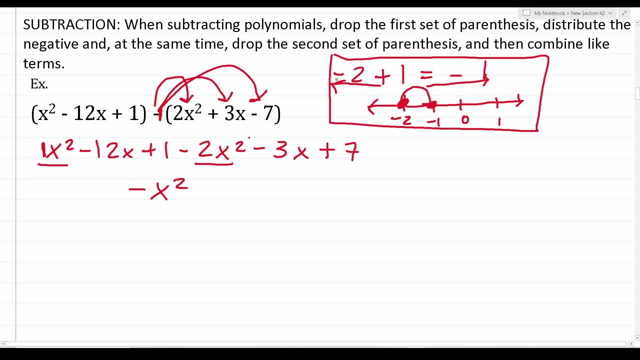 a video about this very shortly. if you need help with adding and subtracting negatives, just bear with me. i'm one guy making videos for the asvab so it takes a little bit of time but i'm going to do it. it takes me a while to get around to covering everything, so with those two like terms, 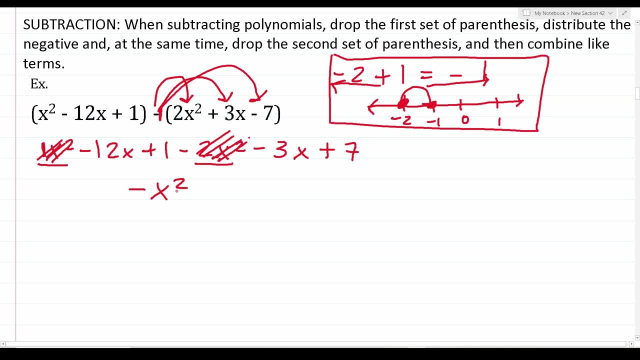 combined. let's go ahead and move on. now we have negative 12x as our next term. again, this is letter variable x raised to the first power. so we're looking for another term with the letter variable x raised to the first power, which is right here. so negative 12x and negative 3x are like terms. 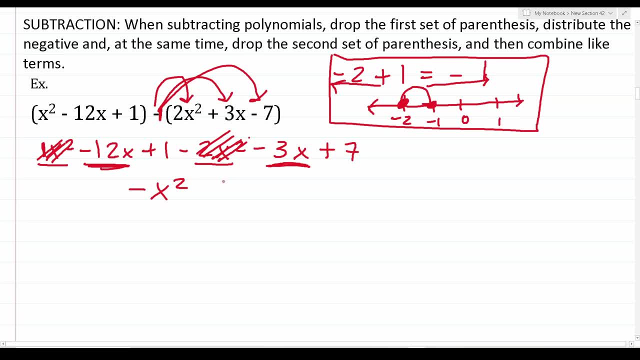 let's go ahead and combine them. negative 12x and negative 3x are like terms, so let's go ahead and combine them. negative 12x minus 3x is negative 12x, negative 13x, negative 14x, negative 15x, and let's 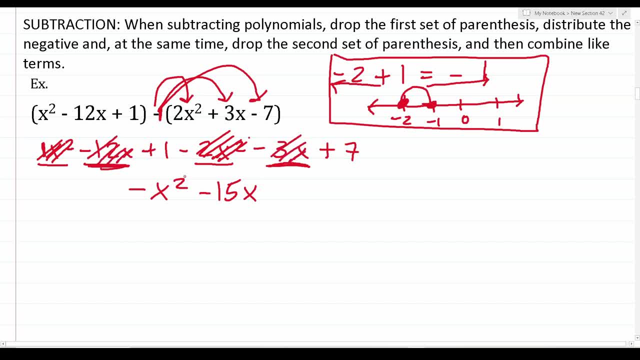 cross them out now that we've combined them, and then finally we have 1 plus 7, which is just 8, right? so that's all there is to subtracting polynomials. again, drop the first set of parentheses. distribute the negative at the same time. drop the second set of parentheses. 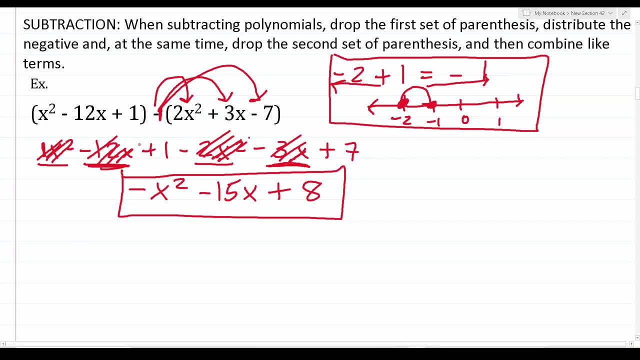 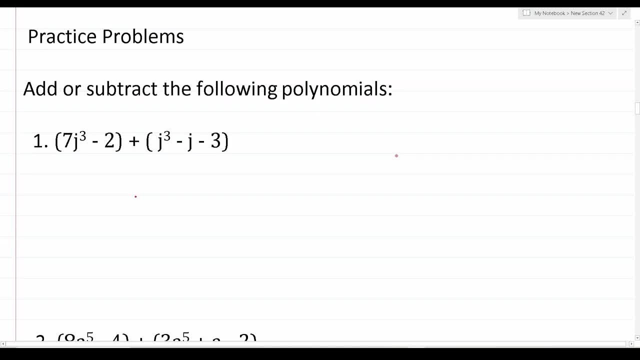 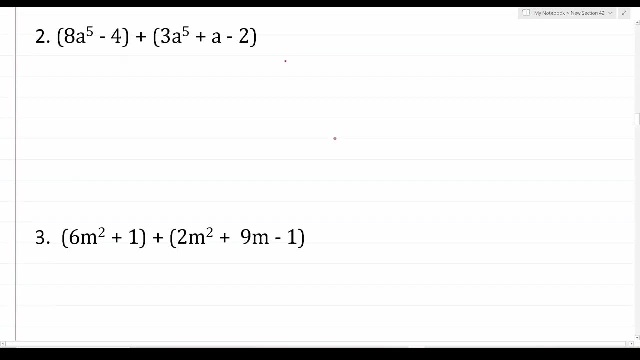 and then combine your like terms, all right? so, uh, that's that one, let's go ahead and move on now. all right, so we've reached the first point in this video, where i would recommend that you attempt to work out the practice problems on your own. uh, there's going to be 10 of them here and none of 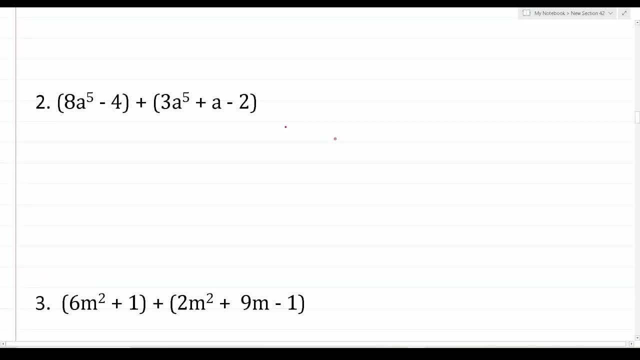 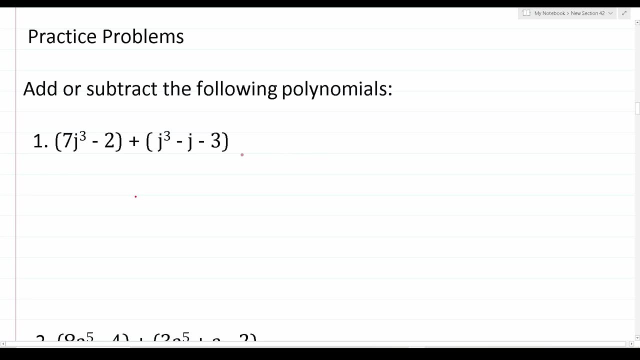 them are too difficult. so, if you'd like, go ahead and pause the video, work out these questions on your own and then resume playing the video to check your solution, um, and then we'll see you in the next video. initially, i'm going to work these out very slowly, but once we get to about question six, 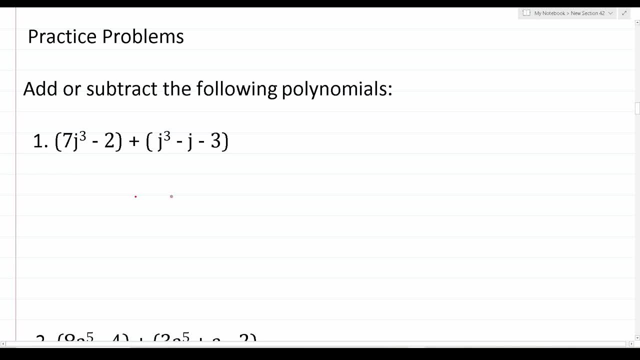 i'm going to start moving very quickly because again, uh, the goal is to give you enough practice in this video such that you're able to do these problems very quickly as well as very accurately. i know i'm saying like terms: same letter, variable raised to the same power. hopefully that becomes. 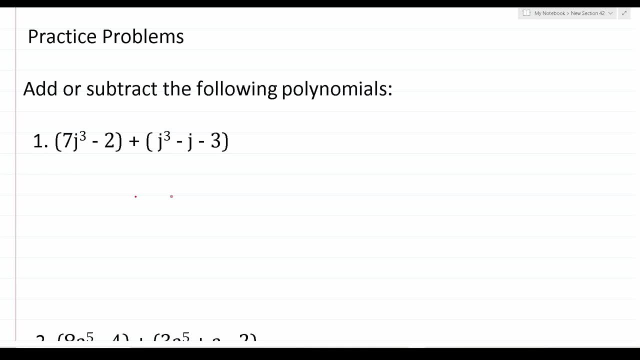 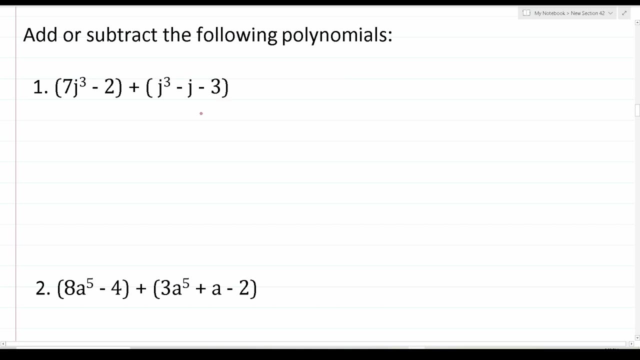 second nature to you, where you can decide if something is a like term with something like that else or not, almost instantly. so with that in mind, let's get uh through these practice problems here, all right. so this uh first question says seven j to the third minus two plus j to the third minus j. 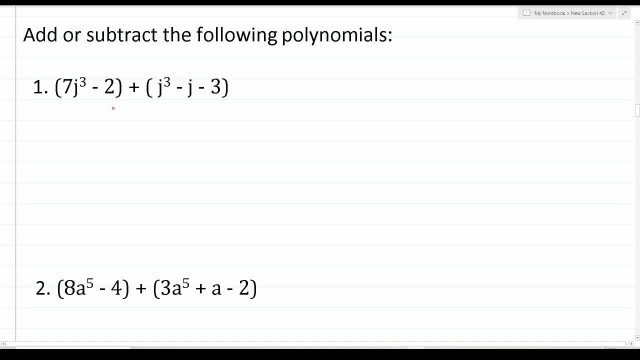 minus three, in case it's helpful. uh, you can say that we're adding a binomial to a trinomial. again, a binomial is a two-term polynomial and a trinomial is a three-term polynomial. but that said, our first question is: what is a binomial and what is a trinomial? 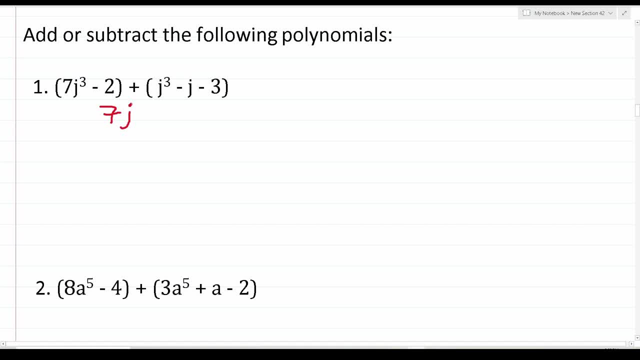 the first step here is going to be to drop the parentheses, so this becomes seven j to the third minus two plus j to the third, minus j minus three. all right, let's combine like terms now. um, our first term here is seven j to the third. if we're looking for its like term, we're looking for 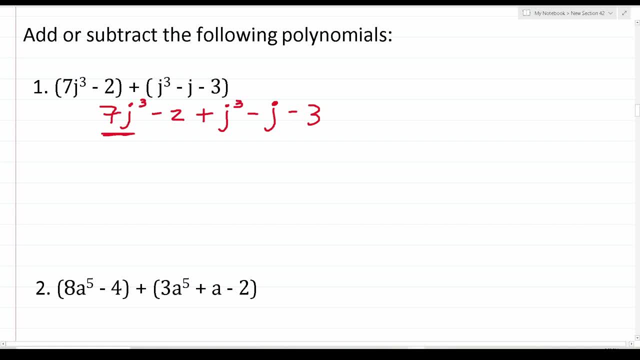 a term that has the same letter, variable j raised to the same power of three. and if we look through our first term, we're going to have a term that has the same letter, variable j raised to the same power of three. and if we look through our other terms, we can see its like terms right here. 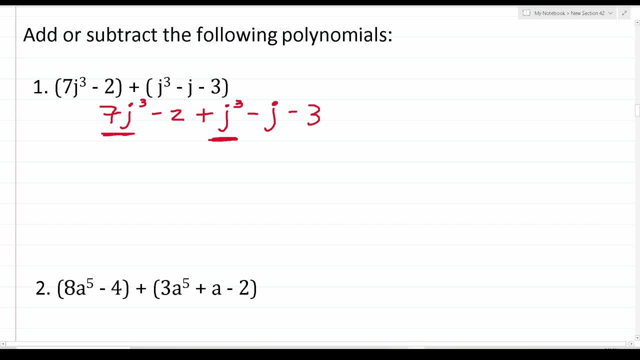 again we have the same letter, variable j raised to the same power, three. if it's helpful, you can place a one here and now we can combine them. seven j to the third plus one j to the third is going to be eight j to the third, and now that we've combined them we can go ahead and cross them out. 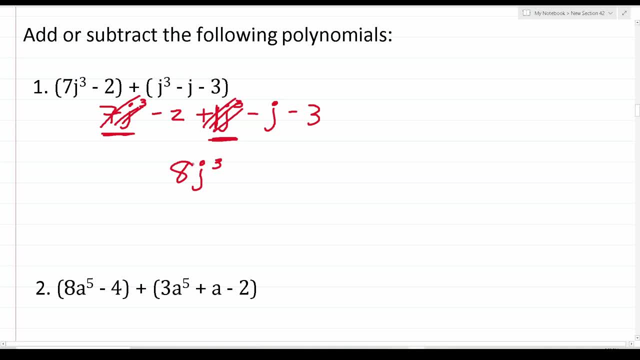 let me stress this: um. order is important when you're simplifying these polynomials, and the way you want to order them is like this: you want the term with the highest uh exponent first, after that you want the uh term that has just a uh letter variable and then, at the very 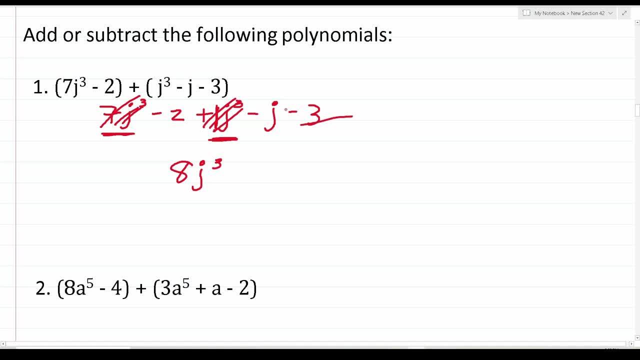 end you can put your whole numbers. so in this case we can see that next we have the whole number negative two. but that said, we still have this letter, variable j. this j is always going to be, always going to come before a whole number, so let's work with it. next, and again we have the 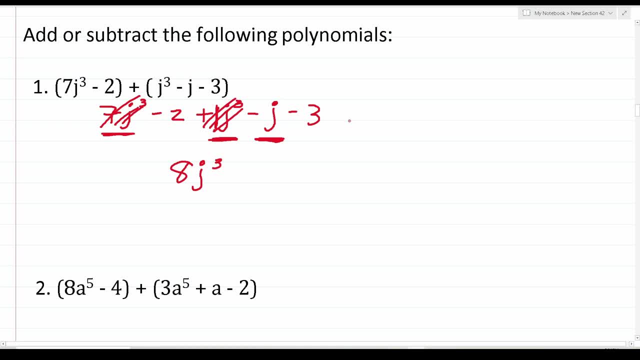 letter, variable j raised to the first power. if we look through the rest of our terms, we can see that none of them are like terms, so we're just going to bring it down accordingly, and now we can cross it out. and then finally, we have negative two and negative three, which is negative five. all right, 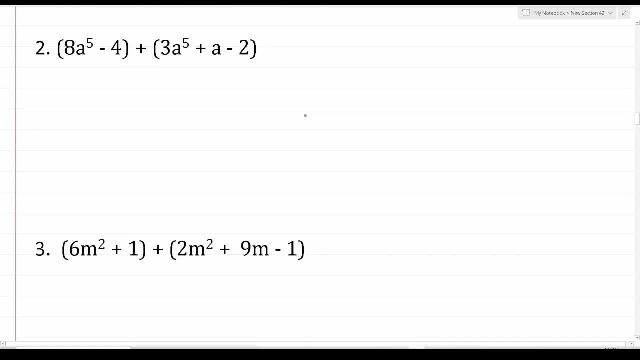 so that's the first one. nothing too difficult there. let's go ahead and move on to the next one. again, we have a binomial that is a two-term polynomial, plus a trinomial that is a three-term polynomial. so let's go ahead and drop these parentheses and combine our like terms. so we have. 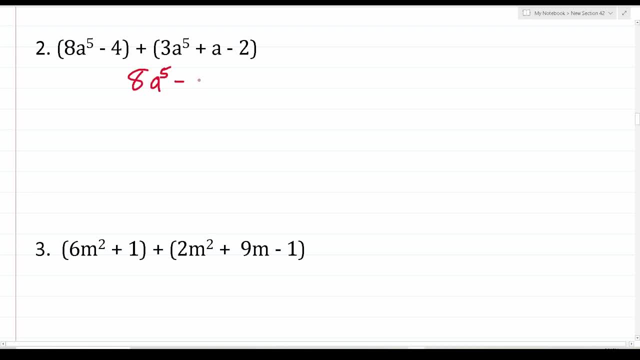 eight a to the fifth minus four plus three a to the fifth plus a minus two. let's start combining our like terms again. we're going to start right here with eight a to the fifth. again, we're looking for another like term, which means we're looking for another term that has the variable a raised to the fifth. and if we 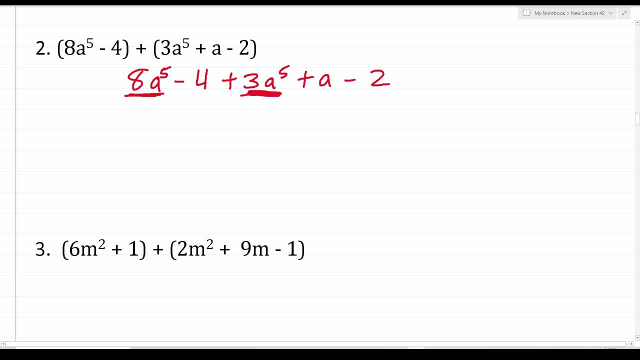 look, we can see that the only other one is right here: a to the fifth. and so we're going to combine eight a to the fifth with three a to the fifth to make that eight, nine, ten, eleven a to the fifth. and now that we've combined those, we can cross them out. 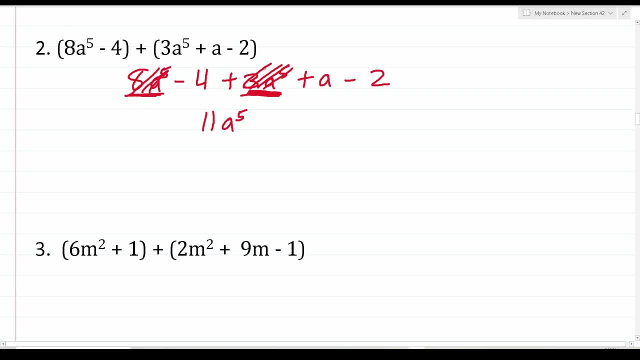 as we saw previously, order does matter. so instead of working on these whole numbers, next i'm going to move on and move and work on our letter variable a here, and if we look through the rest of the terms we can see there are no like terms with just a. so we'll go ahead and 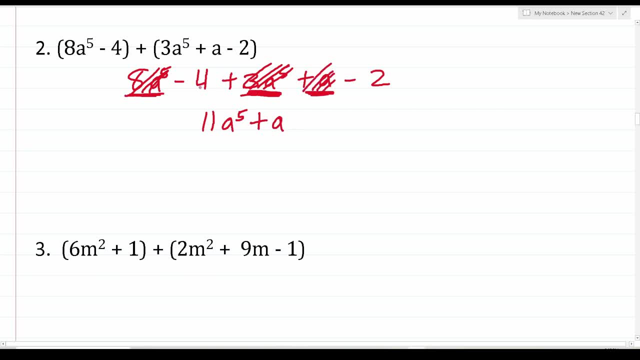 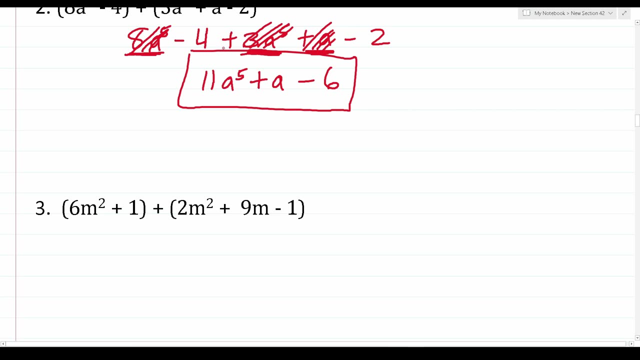 drop that down accordingly and cross it out, and then finally we have, uh, negative four and negative two, and that's going to be negative six. all right, so, uh, that's number two. nothing too difficult there. let me put my box around it to indicate that we're done with it. 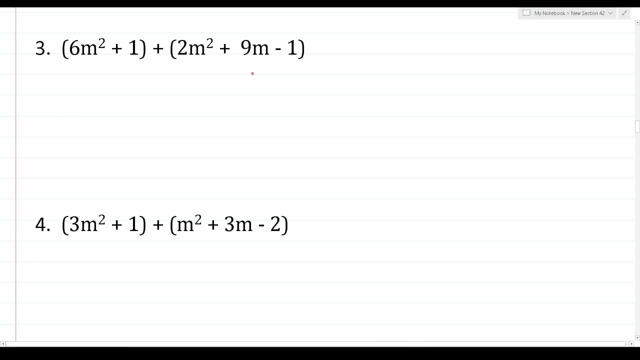 all right. number three says six m squared plus one plus two m squared plus nine m minus one. again, we have a binomial and a trinomial and we're adding those, so let's drop the parentheses. we have six uh m squared plus one, plus two m squared plus nine m minus one. 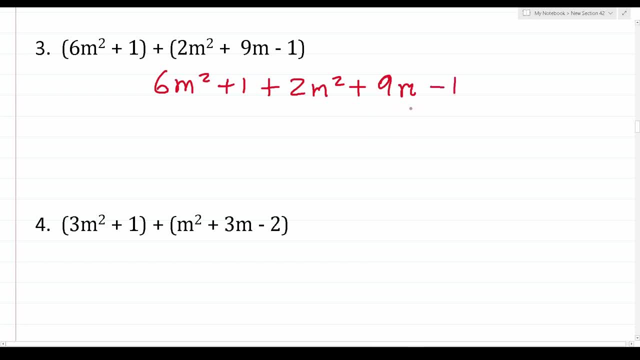 um, now that we've dropped parentheses, let's start combining like terms. let's start right here: we have six m squared, so we're looking for another term that has m raised to the second power. we can see, that's right there. so let's combine six m squared and two m squared to be eight m squared. 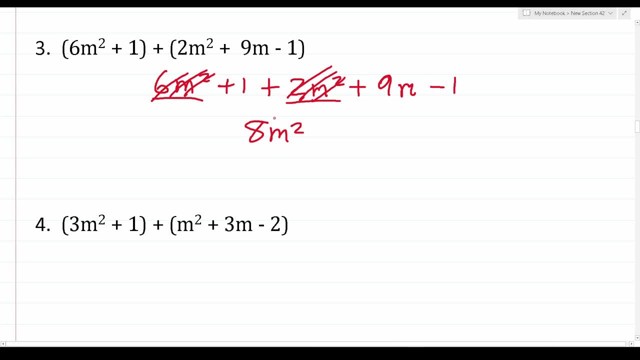 and now that we've combined them, let's cross them out again. uh, a letter variable is going to come before a whole number, so we're going to jump right here to this nine m. we don't see any like terms with nine m, so we'll just go ahead and bring it down accordingly, cross it out, and then we have plus one, minus one, which. 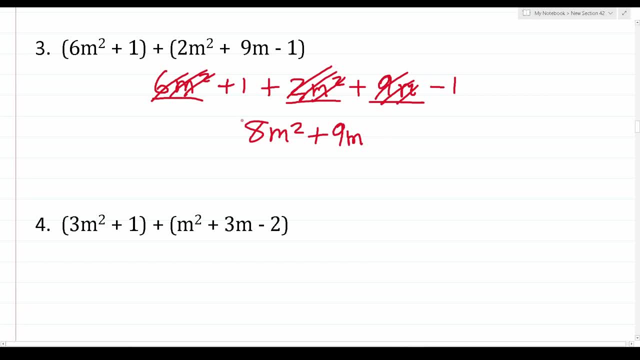 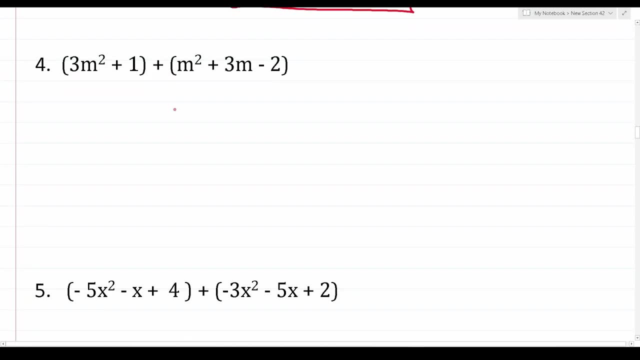 is just zero, and we don't have to write plus zero here. so we're done with this. one number four says three m squared plus one plus m squared plus three m minus two. again, we're just going to drop the parentheses: three m squared plus one plus m squared plus three m minus two. 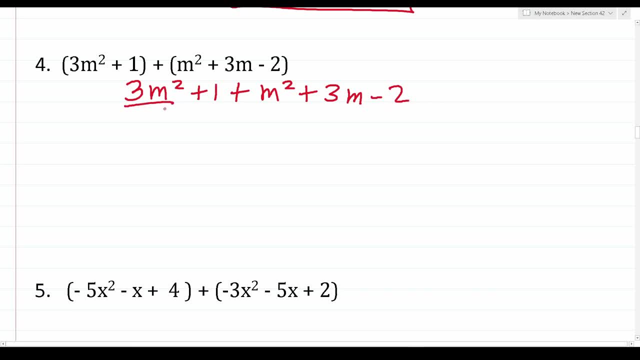 combined like terms now. so if we start right here, we can see that we have the letter variable m raised to the second power, uh, and we can see that we have its like term right here again: letter variable m raised to the same power. and if it's helpful, you can imagine that we can just 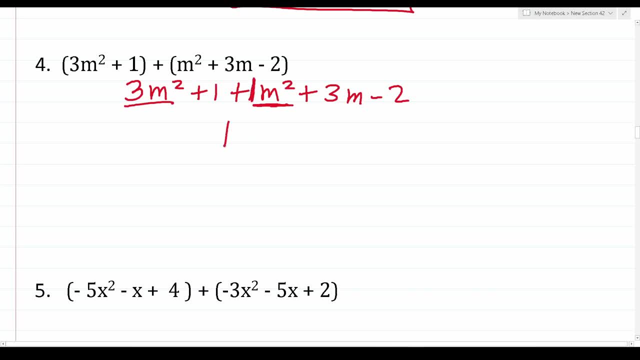 combine the two and we're going to get the same power and then we're going to have a little bit more and there's a one there. So 3m squared plus 1m squared would be 4m squared. We'll cross that out. 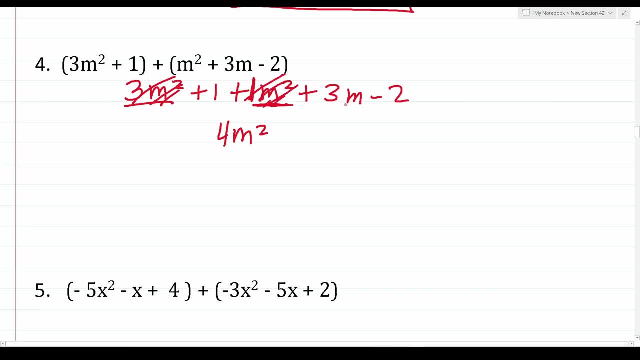 there, And then we have 3m and whole numbers left. So this 3m is going to come next. There's no other like term with it, So we'll go ahead and just bring it down. This will cross out here And then. 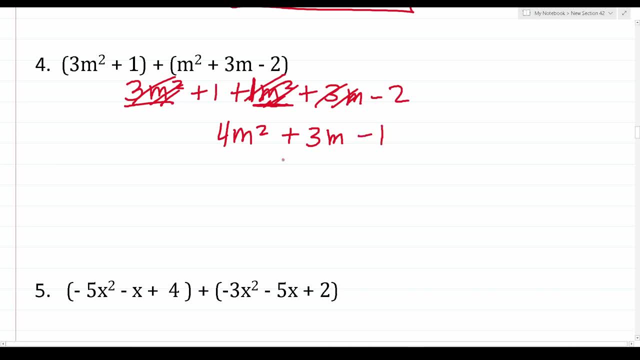 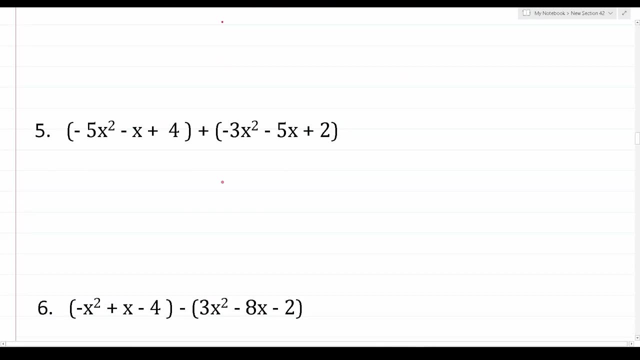 we have 1 minus 2, which is negative 1.. And we are done with that one now. All right, so let's go ahead and work on this one. now Again, we're just adding a trinomial that is a three-term polynomial with another trinomial that is a three-term polynomial, So let's just 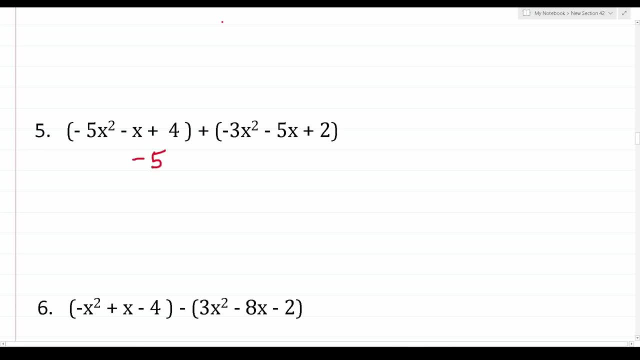 drop those parentheses and combine like terms. So we have negative 5, x squared minus x plus 4 minus 3x squared minus 5x plus 2.. Let's start right here with combining like terms. Again, this is negative 5x squared. So we're looking for a like term of x squared has. 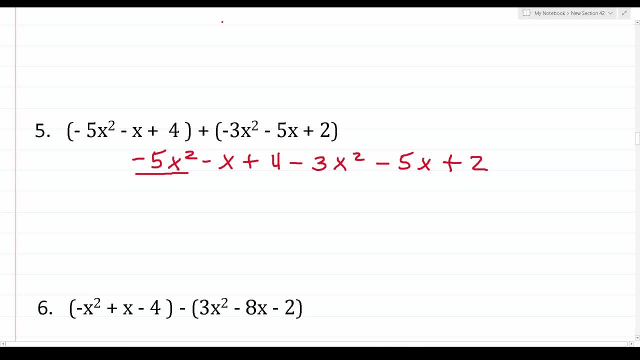 to have the same letter, variable x raised to the same power of 2.. We can see that's right here. That's negative 3x squared. So we can combine those two Negative 5x squared and negative 3x squared is negative 8x squared. 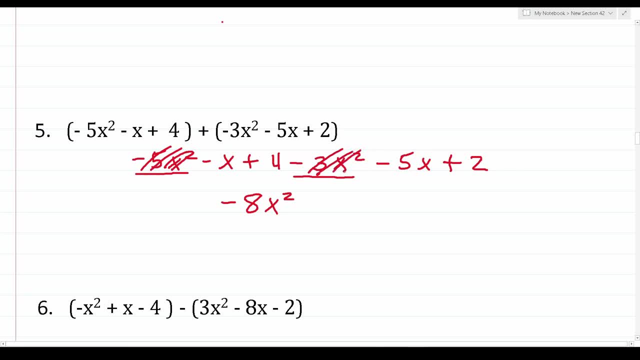 Now that we've combined them, we can cross them out to make this a little bit easier to look at. Next, we have the letter variable x raised to the first power And we can see that it's like term is right here. We have negative x and negative 5x. If we combine those, that becomes negative 3x squared And we can see that it's like term is right here. Now that we've combined them, we can cross them out to make this a little bit easier to look at. Next, we have the letter variable x raised to the first power And we can see that it's like term is right here. And then we have 4 and 2, which is just 6.. Next we have the letter variable x raised to the first power And we can see that it's like term is right here And one of them is negative. so we're going to try to find the right term. 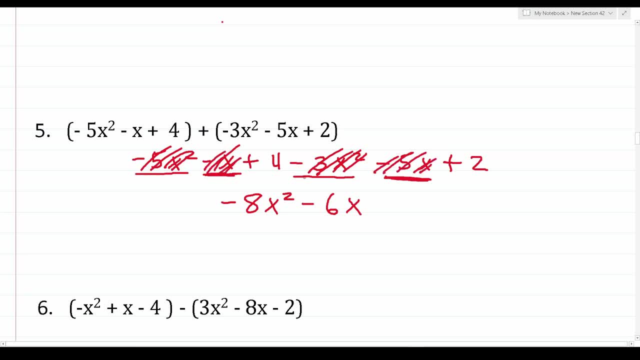 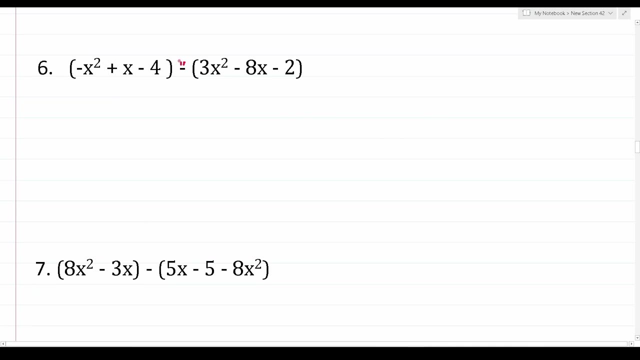 And now we can cross them out, And now we have 4 and 2, which is just 6.. All right, let's go ahead and move on to number 6. now And again. now we have the subtraction, And I don't know why did my pen mark that? 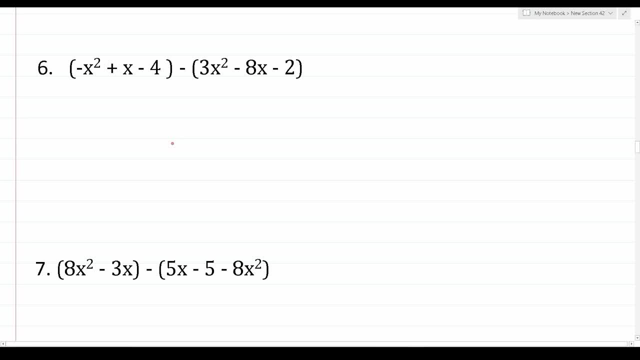 Now we have the subtraction of trinomials. We have this trinomial minus this trinomial. So again, if you recall, the first step is to drop the first set of parentheses. So this becomes negative x squared plus x minus four. After that we're going to take this negative and 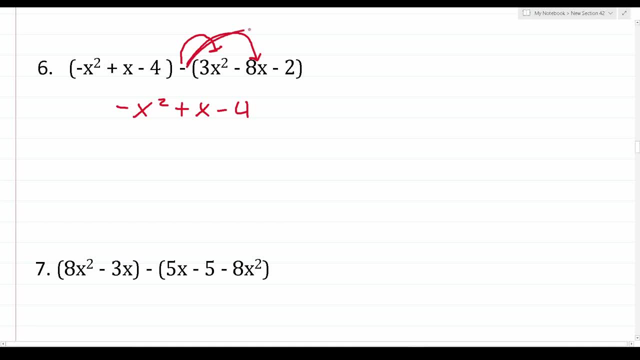 distribute it here, here and here, And at the same time that's going to enable us to drop our parentheses. So again you can imagine there's a negative one here, if that's helpful. but negative times: 3x squared is negative. 3x squared, Again, a positive times, a negative is a negative. Then we 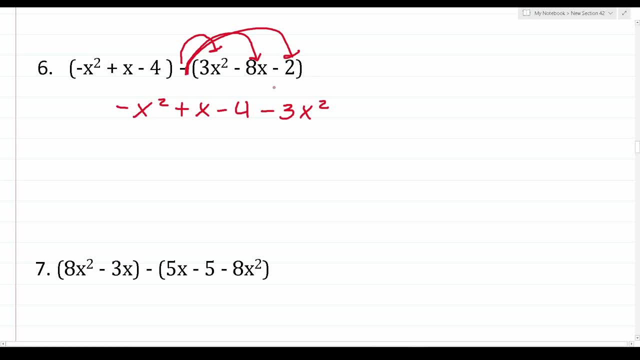 have negative times, negative. 8x. A negative times a negative is going to be positive, So this becomes plus 8x. And then finally, we have negative times, negative, two Negative times, negative is a positive. All right, now that we've gotten rid of our first set of parentheses distributed. 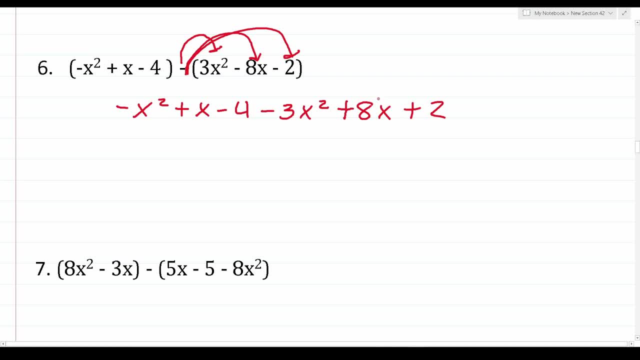 it over here. we're going to take a look at the next step. So we're going to take a look at the this negative and dropped our second set of parentheses at the same time. All we have to do is combine like terms. Our first term here is negative x squared. So we're looking for x raised. 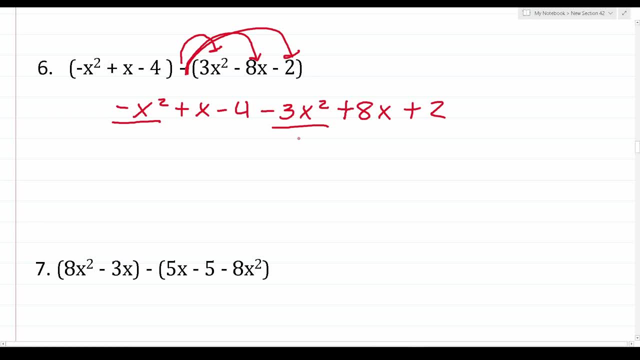 to the second power, which is right here. So negative x squared minus 3x squared is negative 4x squared. Let's cross those out now that we've combined them. Our next term is right here, It's x, and this is technically x raised to the first power. 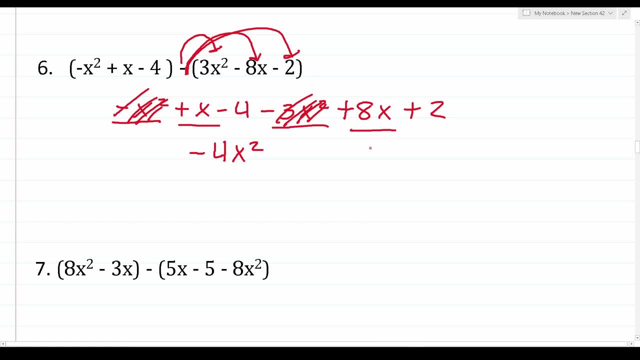 so we're looking for its like term, which is right here. This is 8x, x and 8x again. if it's helpful, put that one there: 8x and x is going to be plus 9x. Go ahead and cross that out. 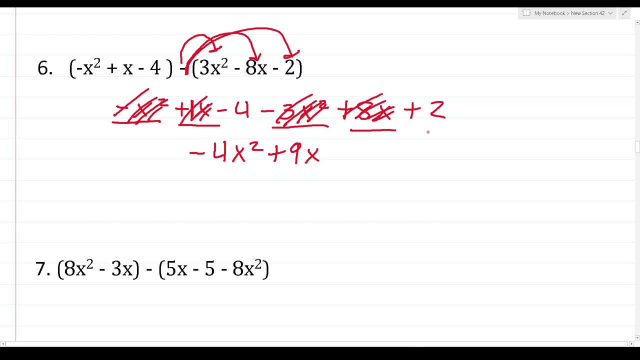 And then finally we have negative 4 plus 2.. Negative 4 plus 2 is negative 2.. All right, so I've noticed that in some of my videos where I work out negatives plus positives, people struggle to do that mentally, So pretty soon. 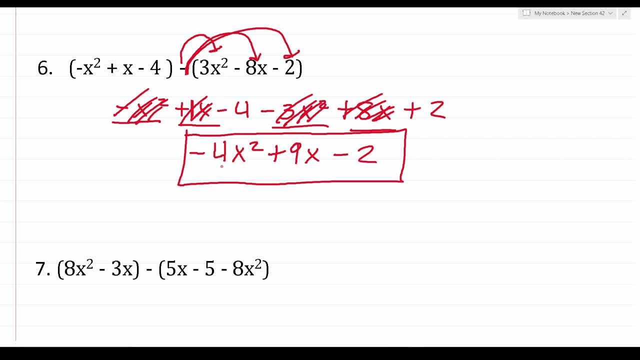 I'm going to create a video in regard to adding and subtracting positive numbers, But, in short, it's actually very easy to do if you visualize these numbers on a number line. So here we had negative 4 plus 2. And let's go ahead and make a nice little number line here, And let's make a 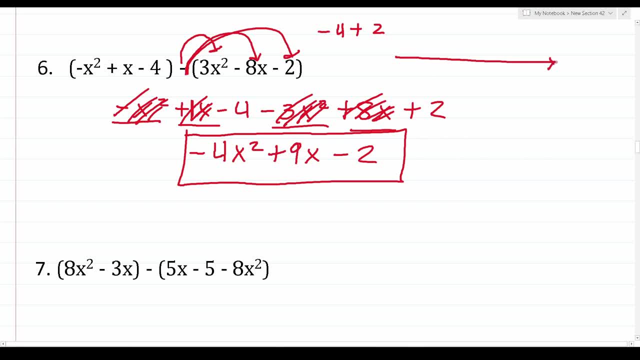 better number line than that if we would. And again, we're going to start at negative 4, negative 3, negative 2, negative 1, 0.. All right, so on a number line, when you move to the right, that means you're adding. When you move to the 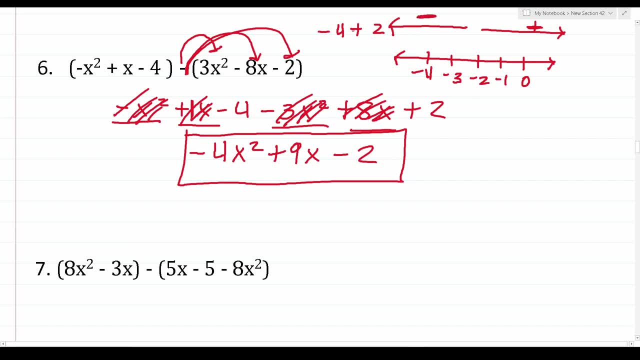 left. that means you're subtracting. So let's start at negative 4, which is right here, And then we're adding positive, or we're adding 2, which means we're subtracting. And then we're going to go to the right two places, 1, 2.. And that's how we get to negative 2.. Okay again. 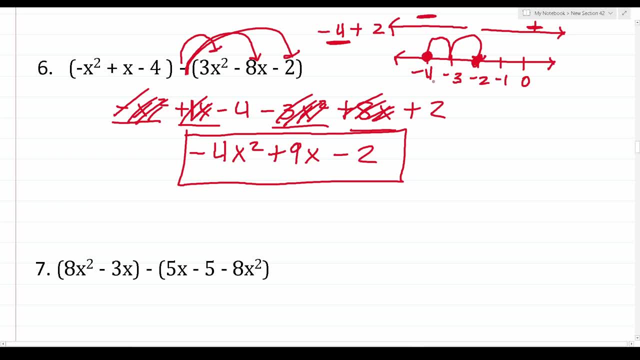 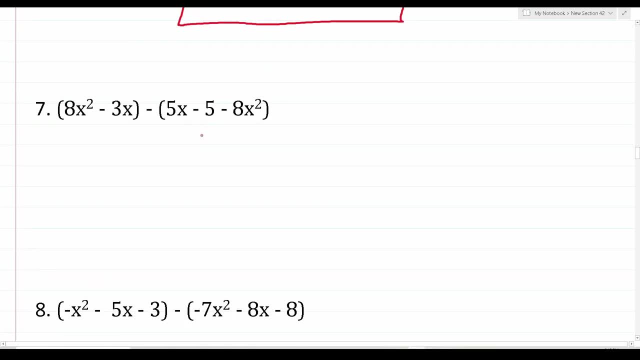 I'm going to make a video on that very shortly, But I just wanted to mention that in case you got lost doing that mental math there. All right, so number 7 says 8x squared minus 3x minus 5x, minus 5 minus 8x squared. As you can see, we're taking this binomial and subtracting it by a. 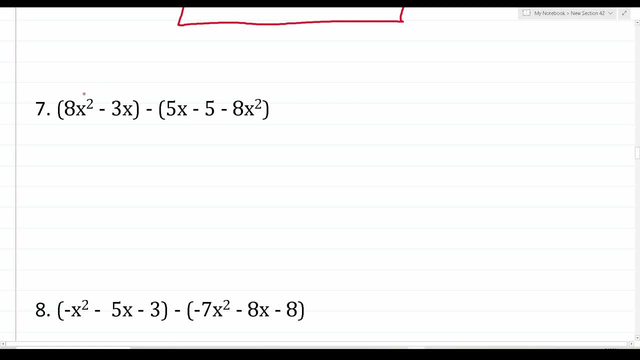 trinomial. And so, if you may recall, our first step is to drop our first set of parentheses, such that this just becomes 8x squared minus 3x. Now we're going to take this negative and distribute it here, here and finally here. Negative times: positive is going to be negative. 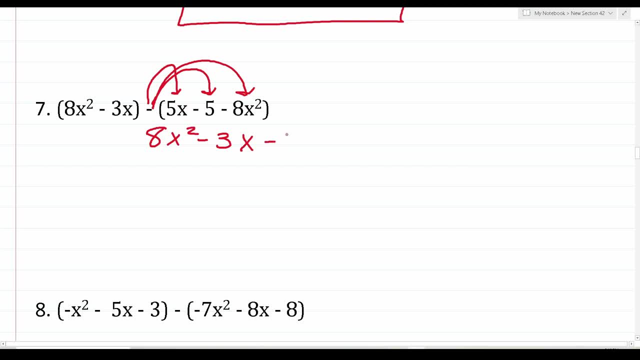 So negative times: positive 5x is going to be negative 5x. Negative times: a negative is going to be a positive. So negative times: negative 5 is just going to be positive, 5.. And then, finally, a negative times: a negative is going to be positive. 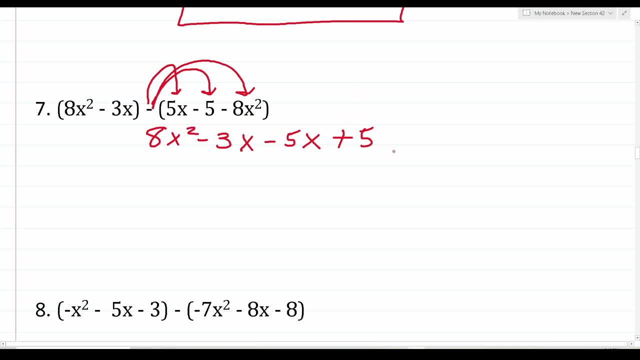 So negative times: negative 8x is going to be plus 8x squared. Let's start combining like terms now. Let's start over here Again. we can see that we have 8x squared. Our letter variable is x, It's. 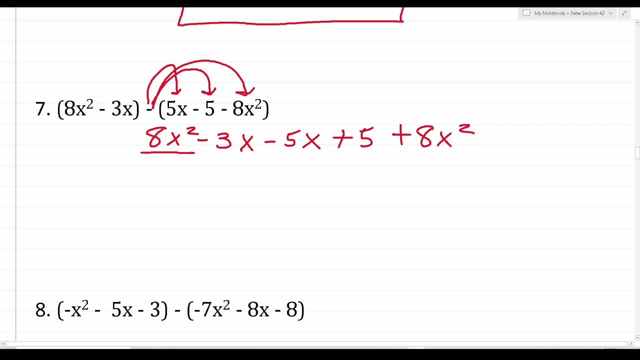 raised to the second power. So if we look through all these other terms, we're looking for x raised to the second power, which we can see is over here. So we can combine 8x squared and 8x squared. That's going to be 16x squared And we can cross these out now that we've taken care of. 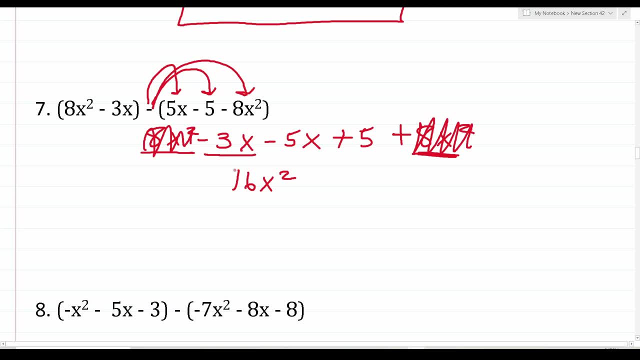 them. Next we have negative 3x. Again that's x raised to the first power. So any other like terms is going to be x raised to the first power And we can see that's right here. So let's combine. 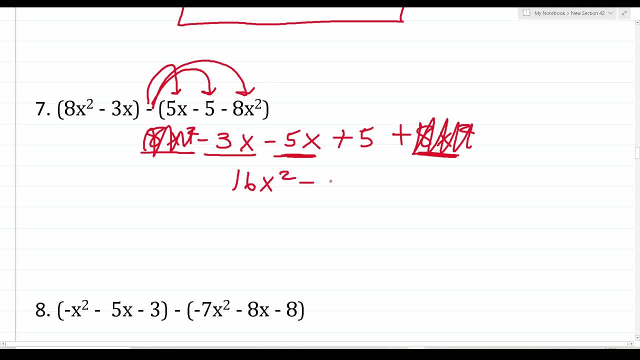 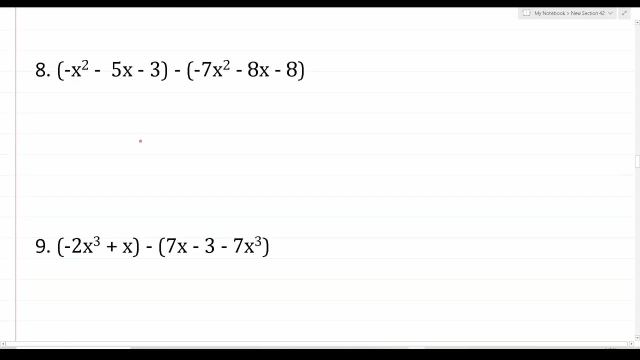 those two Negative 3x minus 5x is negative 8x, And then finally we just have 5.. All right, so that's that one. Nothing too difficult there, All right. so now we have a trinomial minus a trinomial Again, if you recall. 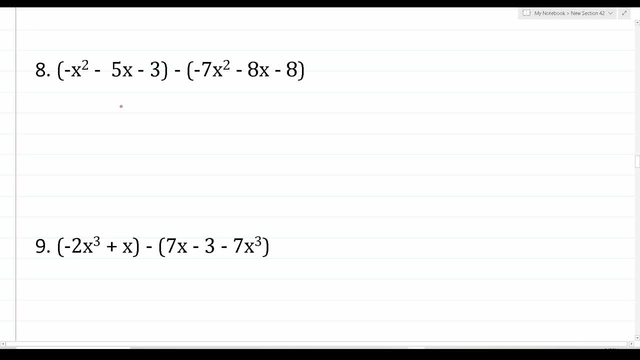 the first step is to drop our first set of parentheses. So this is going to be negative: x squared minus 5x minus 5x squared. Then we're going to take this negative and distribute it here, here and here, And at the same time we do that, we're going to drop our parentheses. 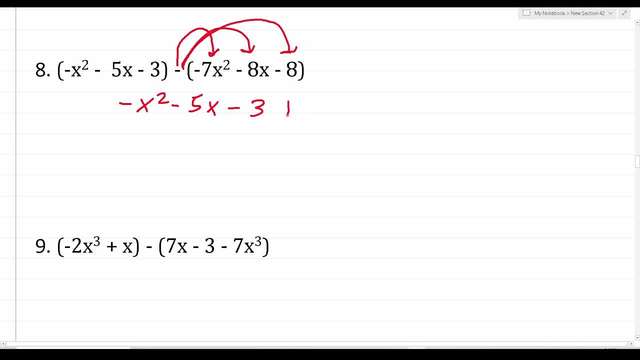 So negative times, negative: 7x squared just becomes positive. 7x squared Again a negative times, a negative is a positive. Then we have negative times, negative. 8x. negative times, a negative is a positive. So this is positive 8x. And then finally, 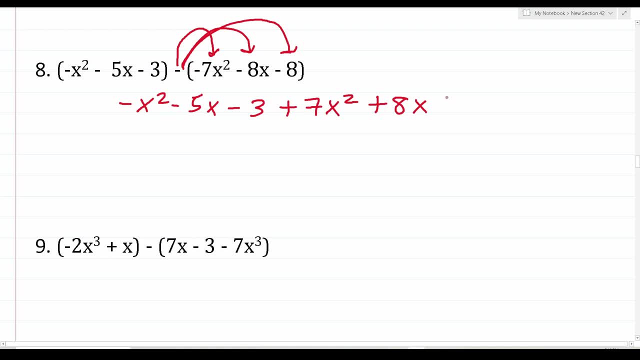 we have a negative times a negative, So negative times. negative. 8 is plus 8.. All right, now that we've distributed that negative and dropped our second set of parentheses, we can go ahead and combine like terms. So we have negative x squared and 7x. 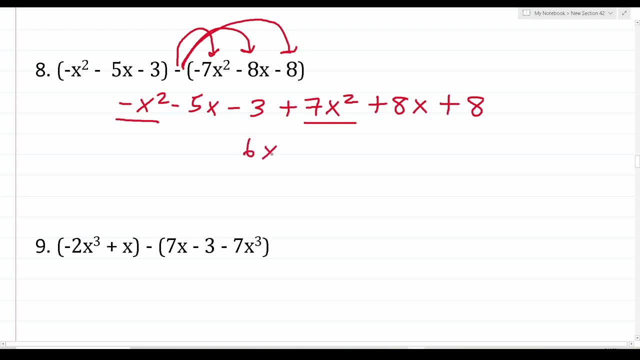 squared, Those combine to be 6x squared, So we'll cross those out now that we've combined them. Then we have negative 5x and 8x. 8x minus 5x is simply going to be plus 3x. 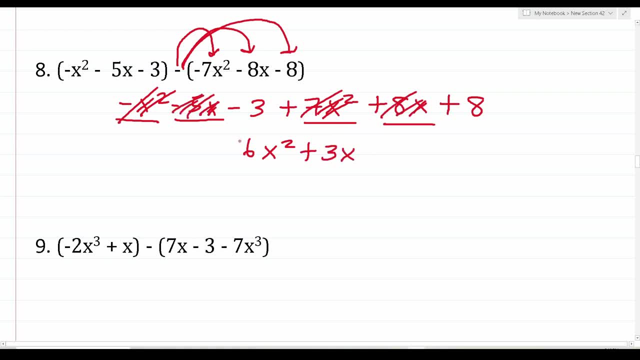 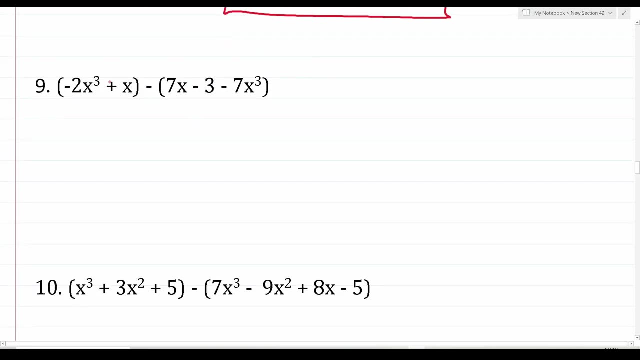 So we'll cross those out. And then finally, we have negative 3 and positive 8.. 8 minus 3 is of course 5.. And there we have it All right. two more to go, All right, so we're subtracting a binomial by a trinomial in this case, So let's drop our first. 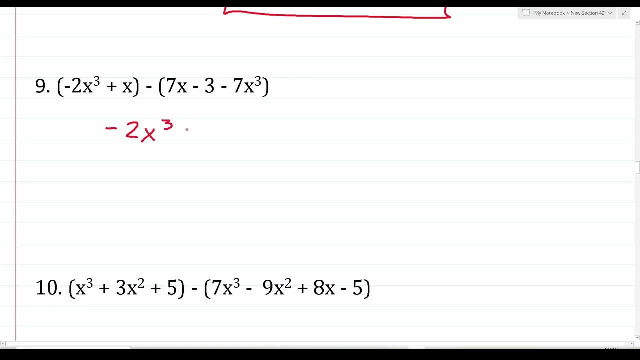 set of parentheses. This becomes negative 2x to the third plus x. Let's take our negative and distribute it here, here and here. So we have negative times positive 7x, That's going to be negative 7x. We have negative times, negative, 3.. And negative times, a negative is a positive, So 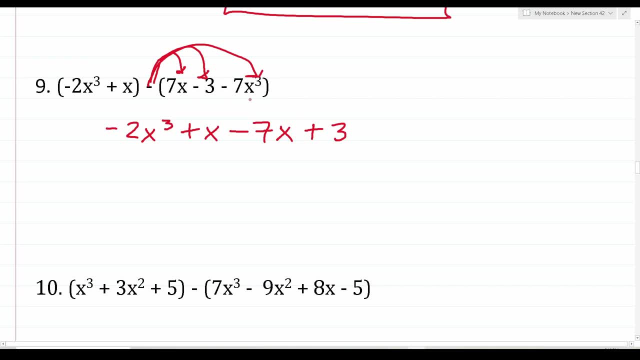 this becomes plus 3.. And then, finally, we have negative times, a negative, So negative times. negative. 7x to the third becomes positive, 7x to the third. Now that we've distributed that negative and dropped our second set of parentheses, we can go ahead and combine those together, So we're. 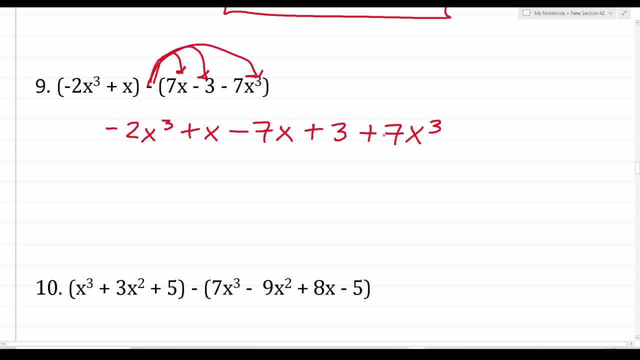 our second set of parentheses. Let's go ahead and start combining some like terms here. So we have negative 2x to the third there and 7x to the third there. Let's combine them to be 5x to the third. 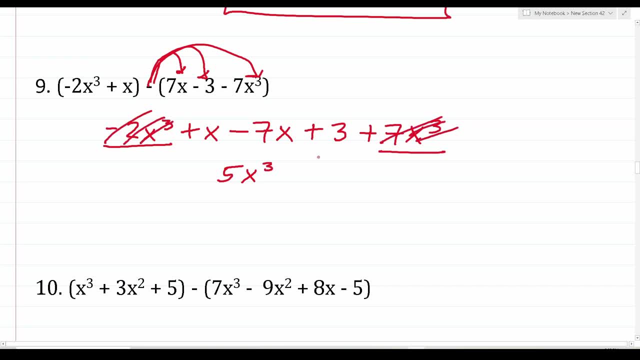 We can cross these out. All right, our next set of like terms is right here: Positive x and negative 7x. Positive x and negative 7x is negative 6x, So we'll go ahead and combine those together And 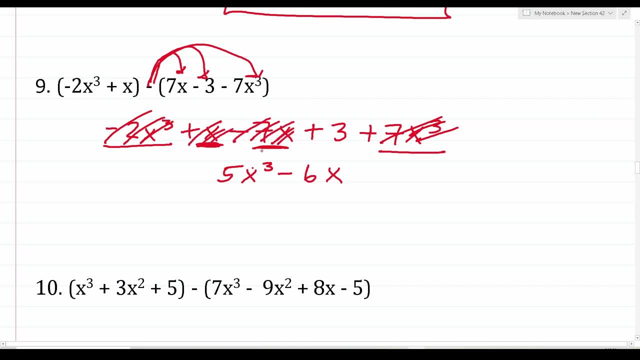 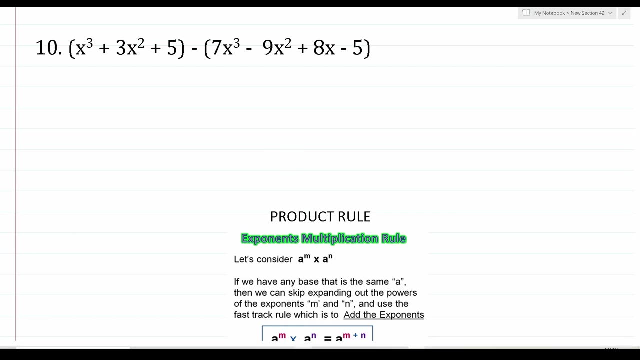 we can cross those out now that we've taken care of them, And then we just have this plus 3 hanging out here. So we'll go ahead and tack that on at the end And we are done with that one, All right. so our last problem is a little more challenging insofar as we're taking a trinomial. 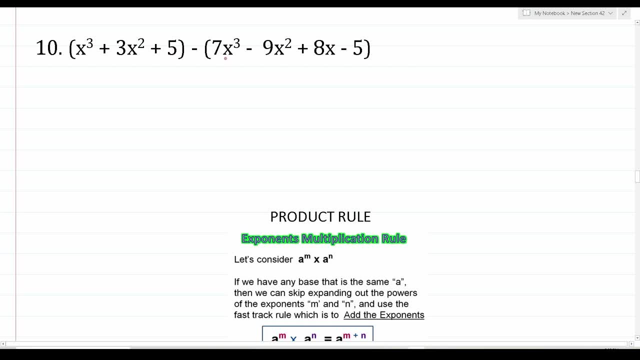 and we're subtracting it by a quadrinomial, That is a four-term polynomial. So process is the same. Drop the first set of parentheses. This becomes x to the third, plus 3x, squared plus 5.. Take our negative and distribute it. 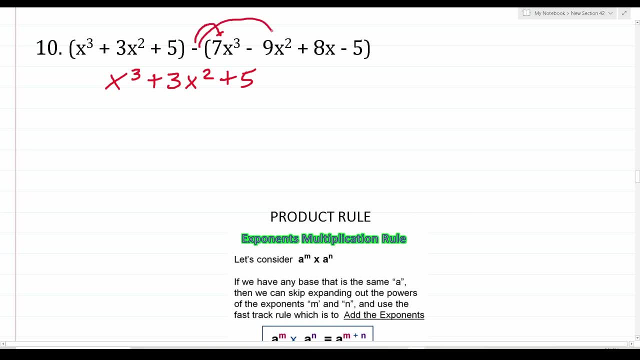 accordingly. So we're going to distribute it here, here, here and here, And at the same time that we're distributing that negative, we're going to be able to drop our second set of parentheses, So this becomes negative times, positive 7x. 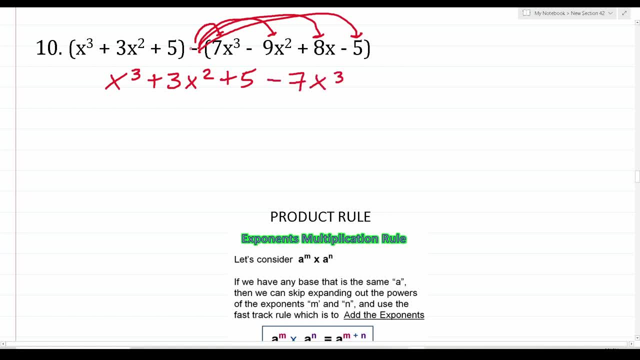 To the third, which is going to be negative. 7x to the third. Negative times: a negative is going to be a positive, So this is plus 9x squared. Negative times a positive is going to be a negative, So this is minus 8x. And then a negative times a negative is a positive, So this is plus. 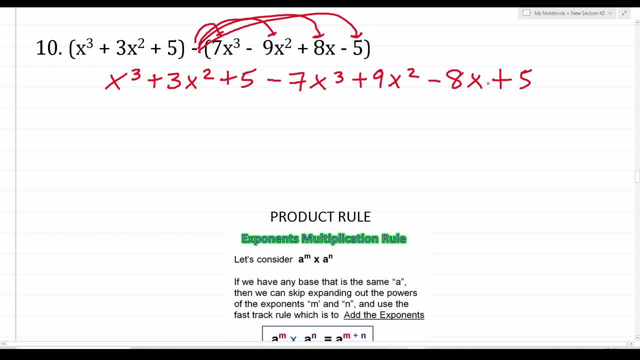 5. Let's go ahead and carefully combine our like terms here. So we have x to the third and x to the third here. Specifically, we have 1x to the third- You can put that one there if you need it- 1x to the third. we have 1x to the third minus 7x to the. 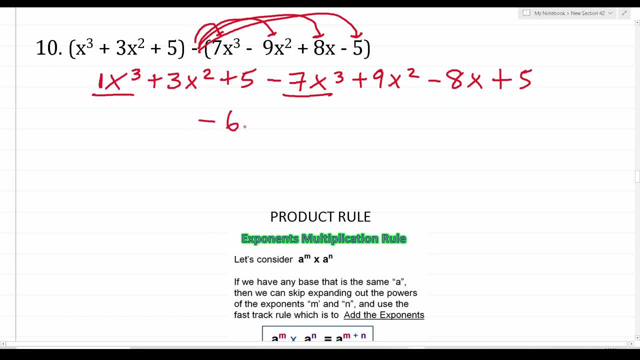 third. so that's going to be negative 6x to the third. Cross those out now that we've taken care of them. Next, we have 3x squared and we can see that we have 9x squared, So let's go ahead and combine those next 9,, 10,, 11,, 12. 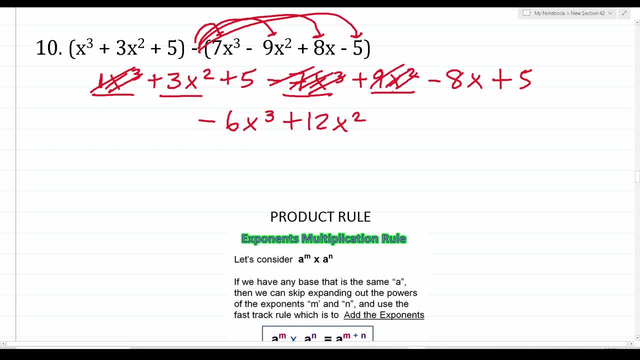 so this is plus 12x squared. cross those out now. and then, before we deal with these whole numbers, we have this uh variable of just x to the first to deal with. so let's bring that down here so that our polynomial is in order at the end. so we have negative 8x, this crosses out. and then finally we have 5 plus 5, which is 10.